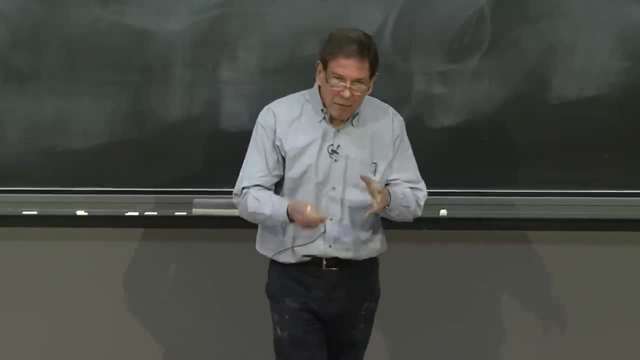 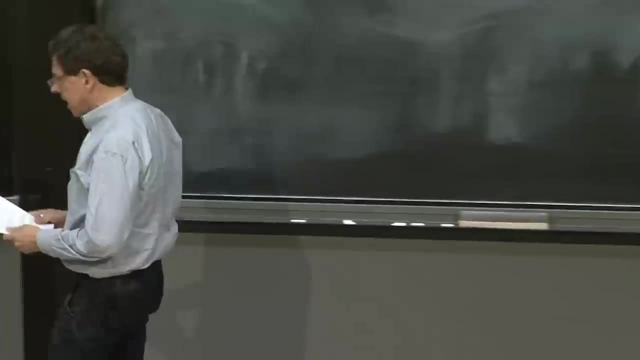 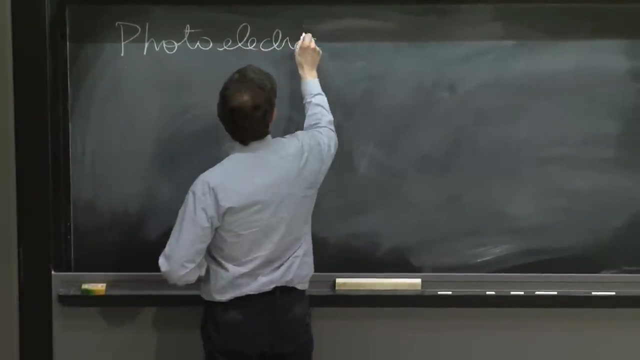 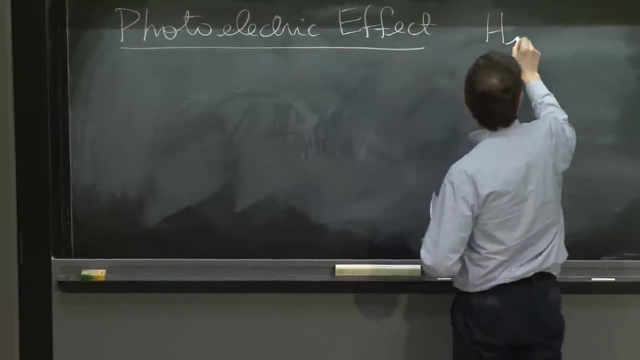 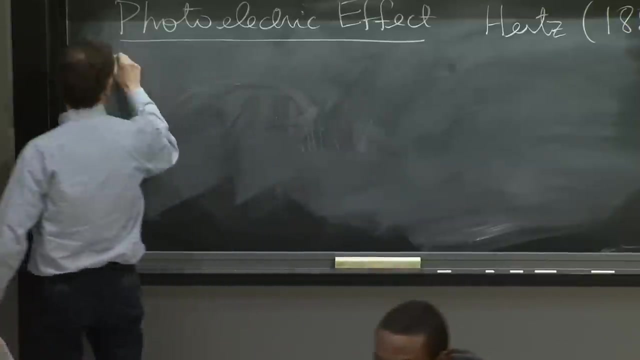 Those were called photoelectrons And therefore you would get a photoelectric current from those electrons. So this is the effect we want to discuss now. It's the photoelectric effect and it's Hertz 1887.. So first the description. 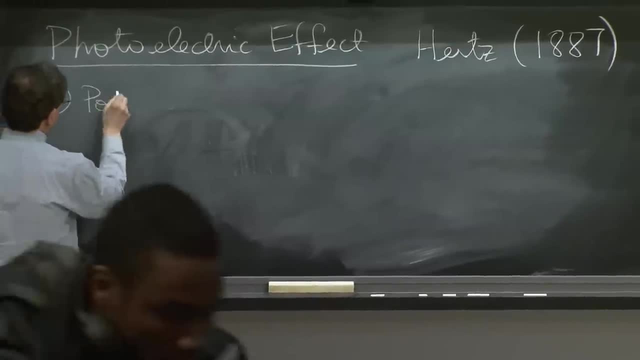 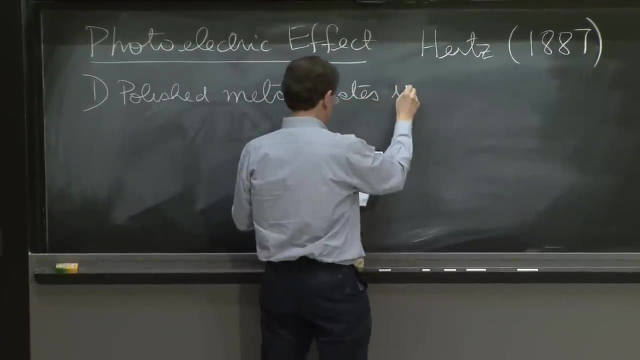 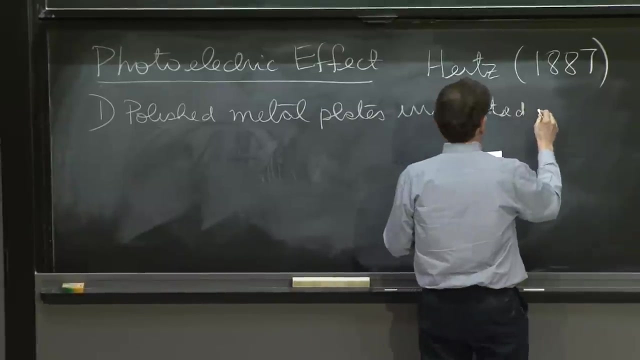 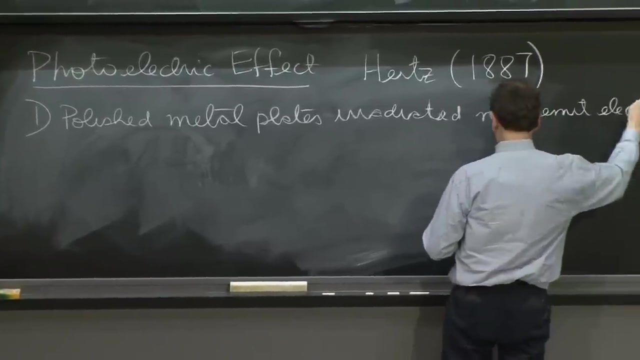 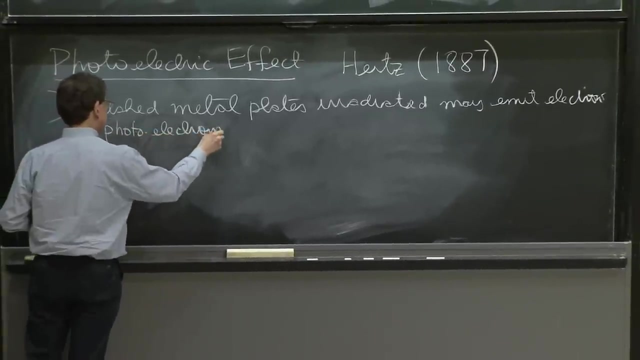 So polished metal plates, Polished metal plates, Etc. Irradiated. Irradiated May emit electrons And these are called photoelectrons, sometimes Photoelectrons. It's just an electron, That wasn't- I forgot. 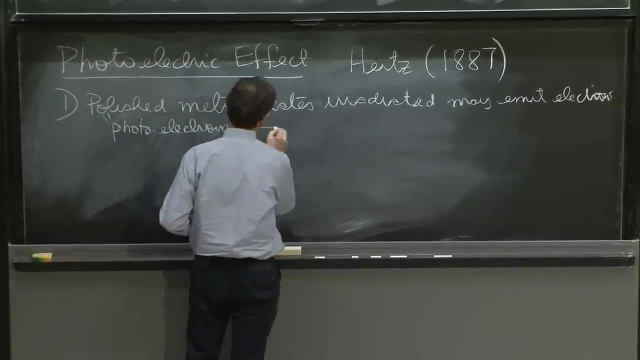 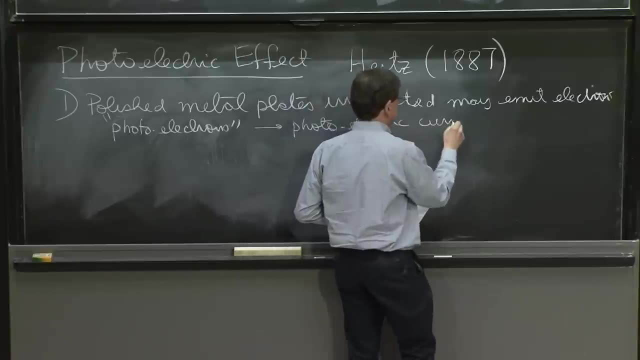 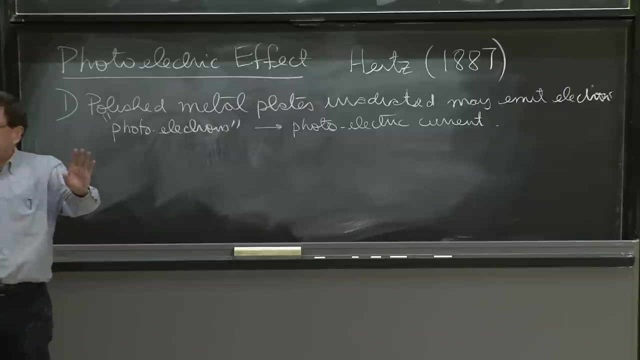 Yeah, was released due to a photon And therefore we get a photoelectric current, photoelectric current. OK, so far, so good. But what was special about this experiment? The first step that was special was that there was a critical frequency. 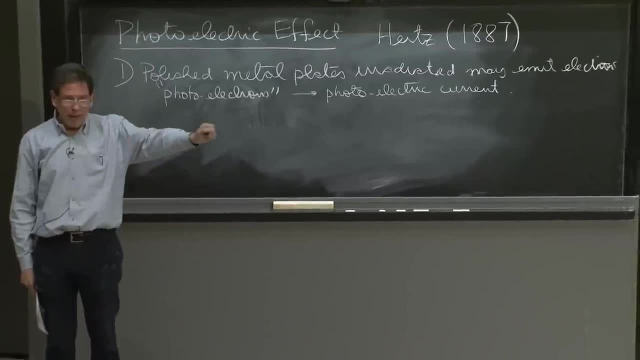 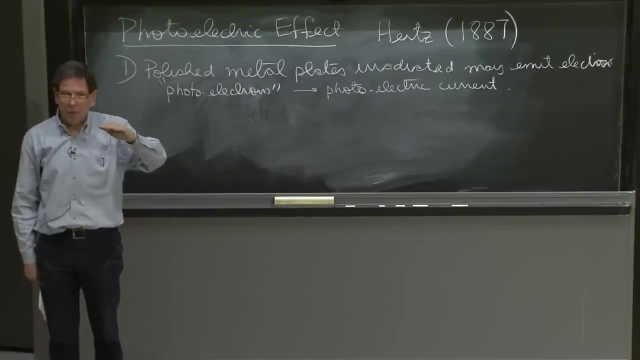 If you would take a sample and you would irradiate it with light, and you would begin with light with very low frequency, nothing would happen. And all of the sudden, after a certain frequency, boom, you would get a current. So there is a threshold- frequency. 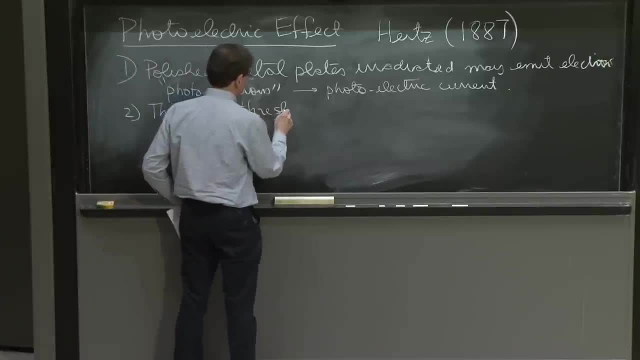 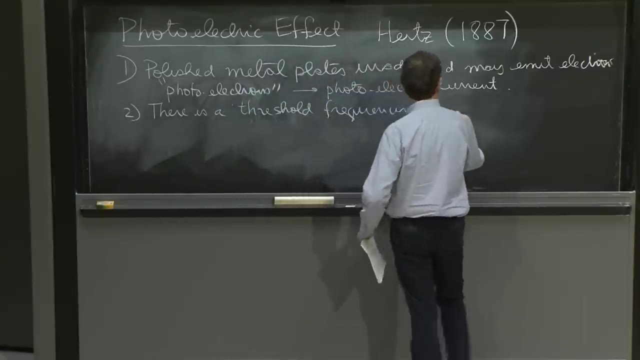 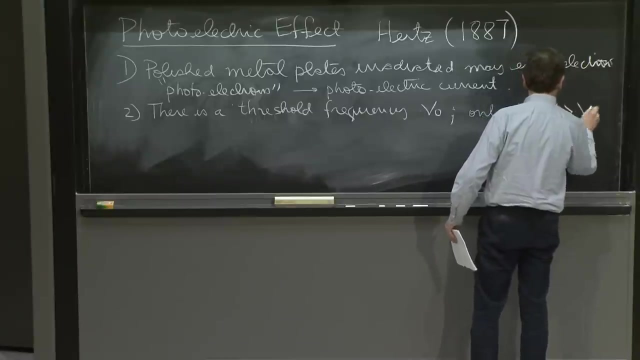 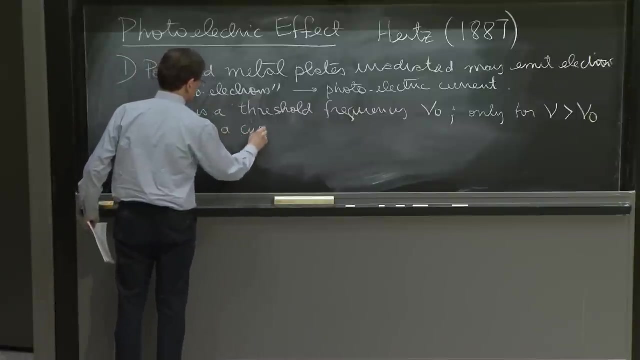 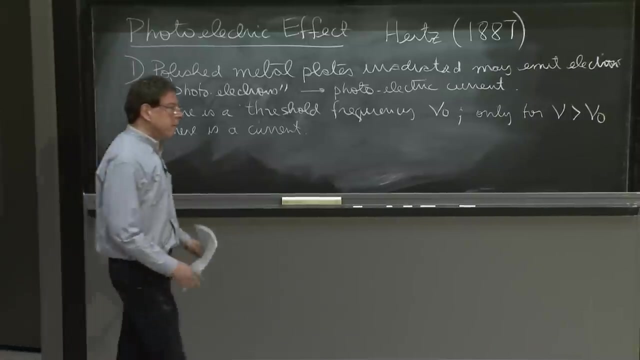 There is a threshold frequency: nu 0.. There is a threshold frequency such that only for nu greater than nu 0, there is a current, So no current for lower frequencies. Now, as it turned out, nu 0 depends on the metal. 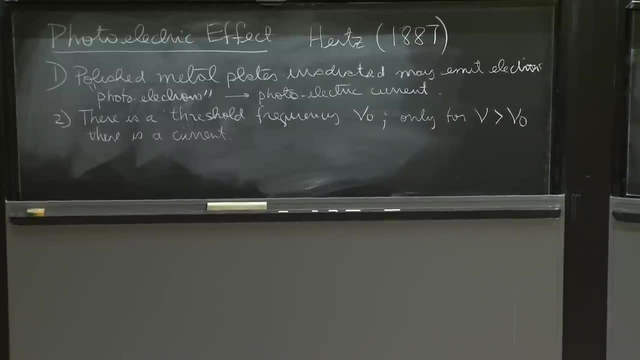 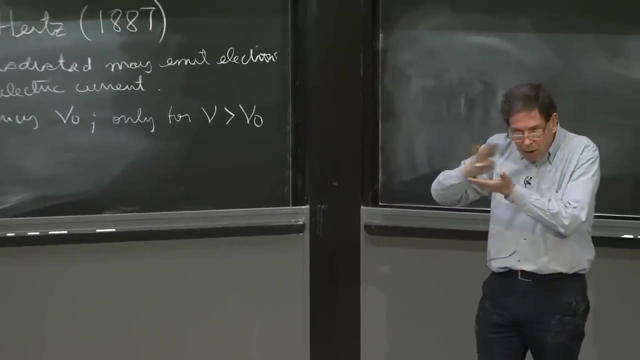 you're irradiating, And even more. It's a complicated thing, OK, OK, OK. So what does that mean? It's a complicated thing to calculate. It depends on the surface of the metal. So that's why Hertz apparently had to polish the metal. 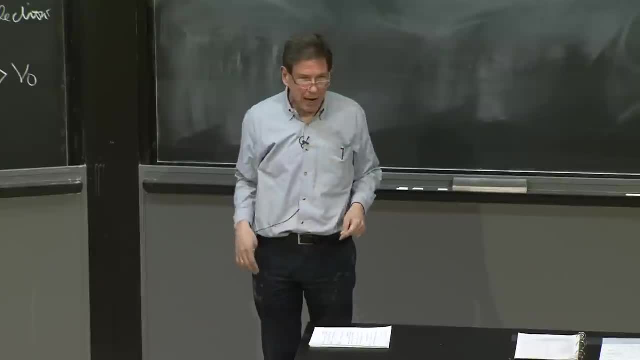 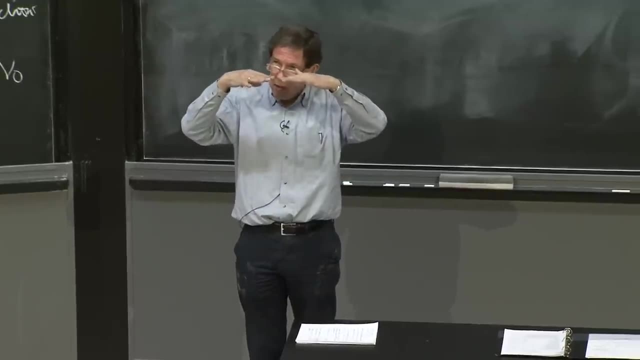 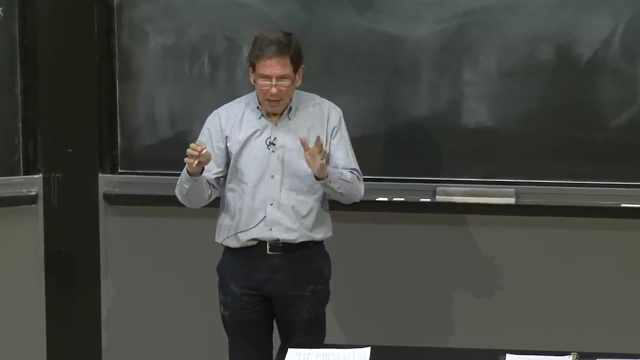 And this frequency, if the metal is irregular, may depend on where you shine. So you better prepare the metal very nicely. And it may even depend on the crystalline nature of the metal, because it's a many body effect. Anticipating the resolution, there is this piece of metal. 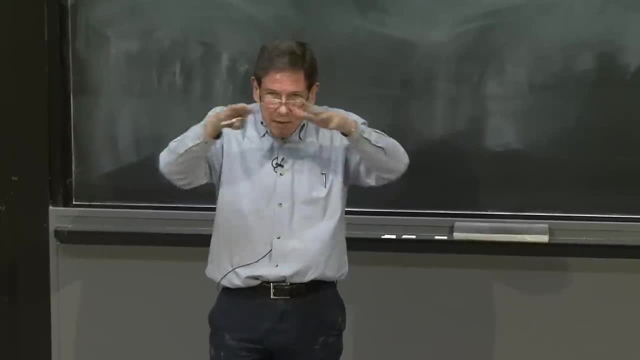 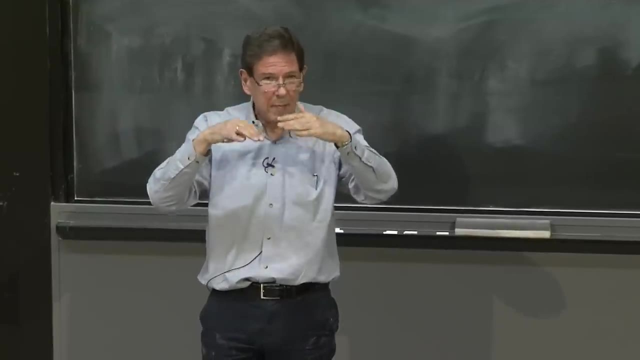 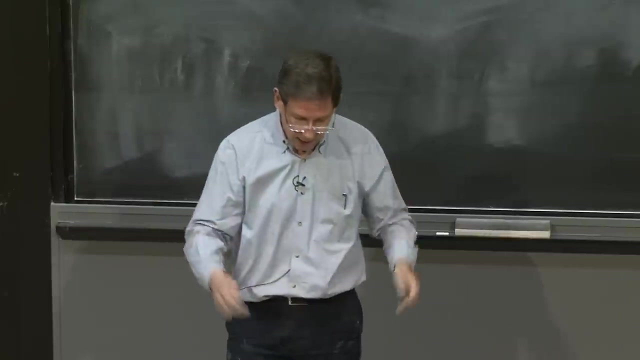 And there are a few free electrons running around And they run around among the crystal, the crystalline structure of the metal, And removing them it's going to take some energy And that energy depends on the metal and the arrangement and all kinds of things. 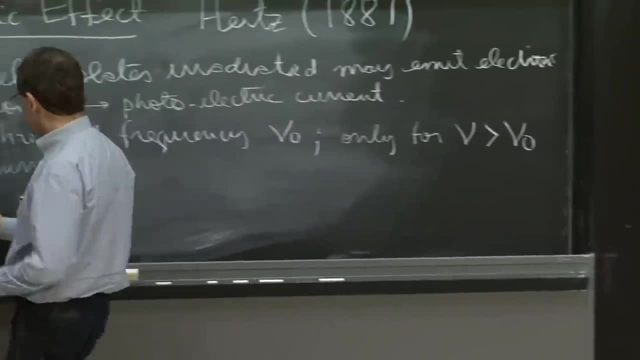 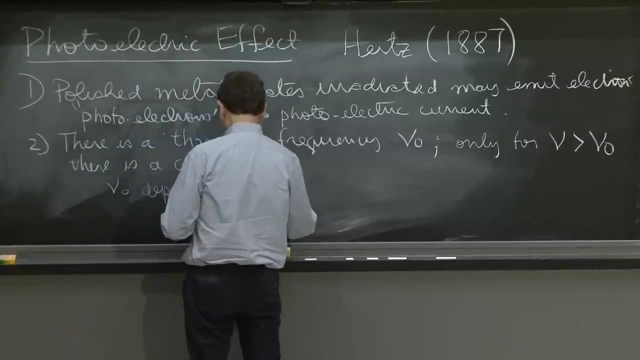 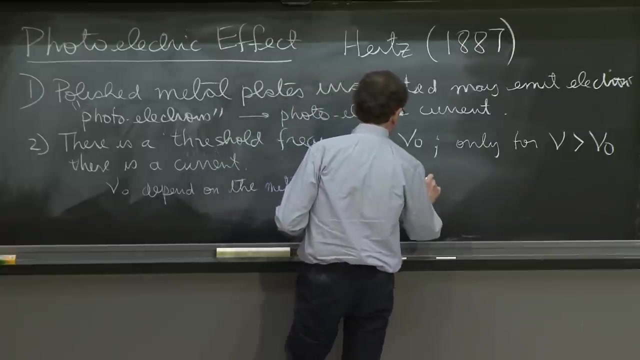 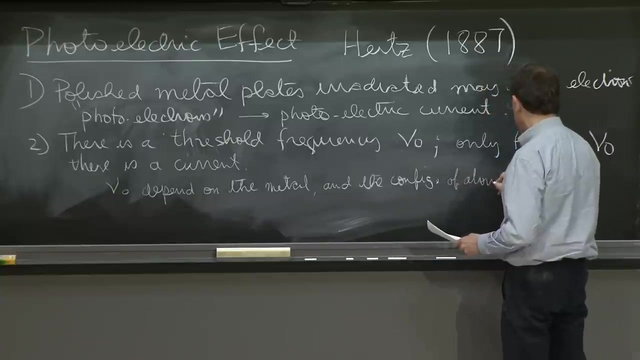 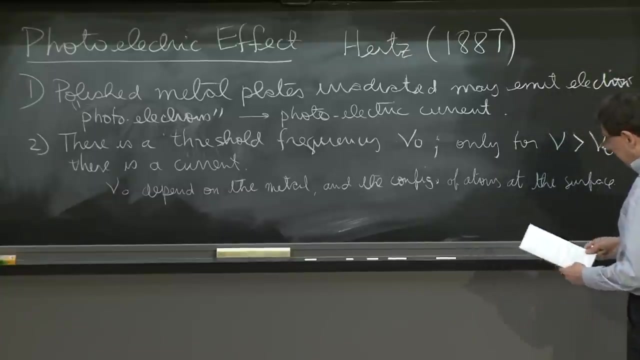 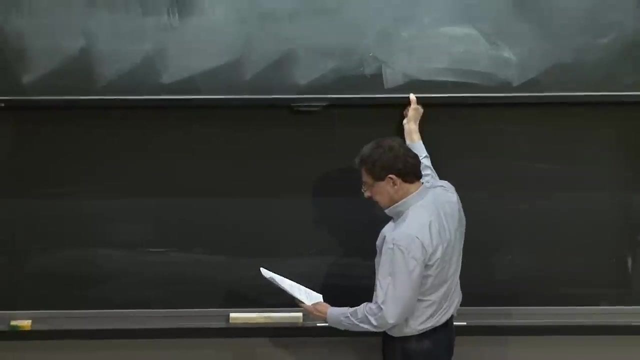 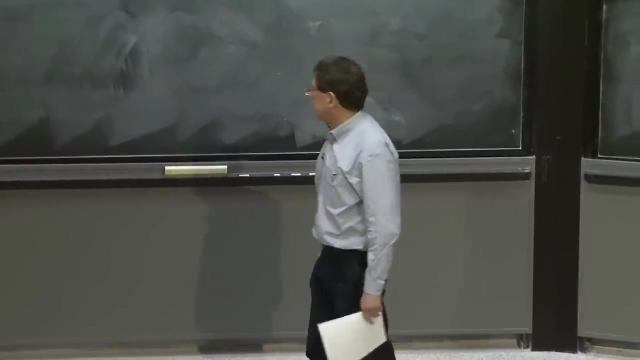 So this mu 0 depends on the metal and the configuration uration abbreviate of atoms at the surface Surface. Third property was kind of interesting. The magnitude of the current was proportional to the intensity of the light Magnitude. 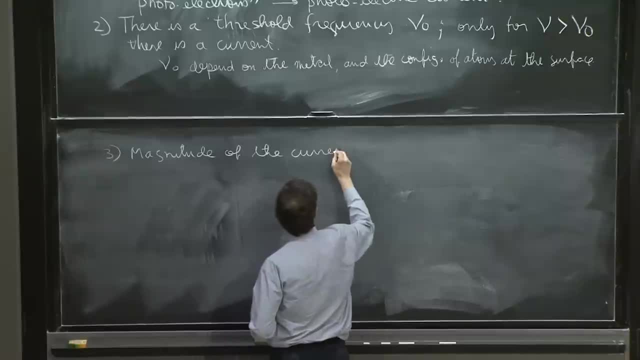 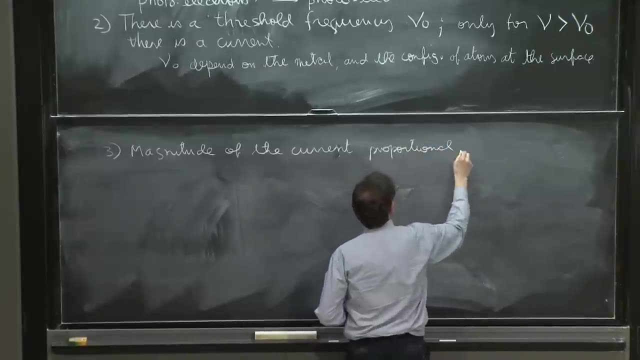 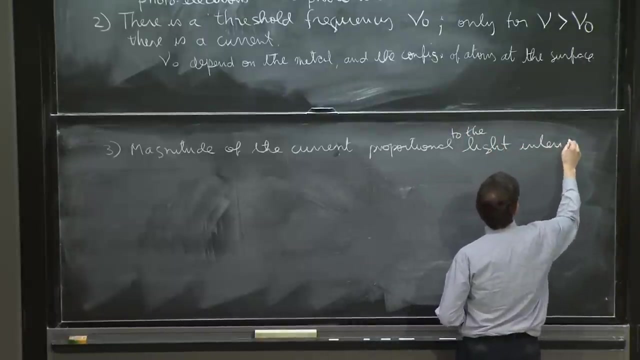 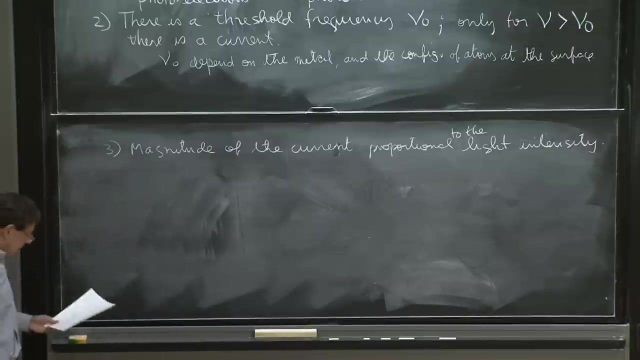 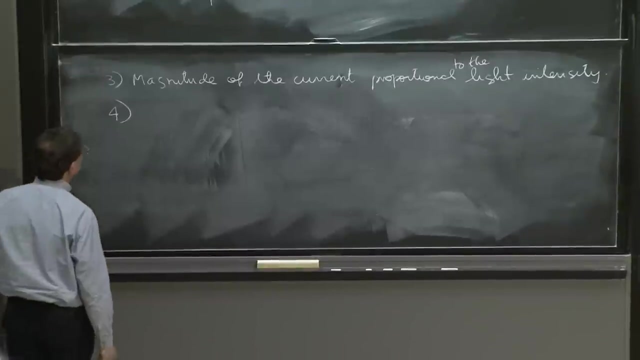 Current. It's proportional to the light intensity. to the light intensity. And perhaps the last one and fourth, a rather important one, a very crucial property is that you could observe the energy of the photon. The energy of the photon is independent of the photoelectrons. 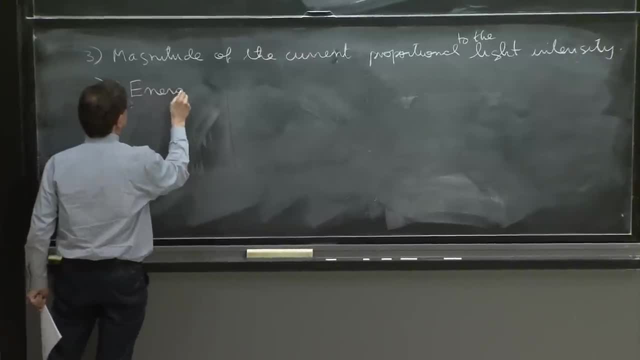 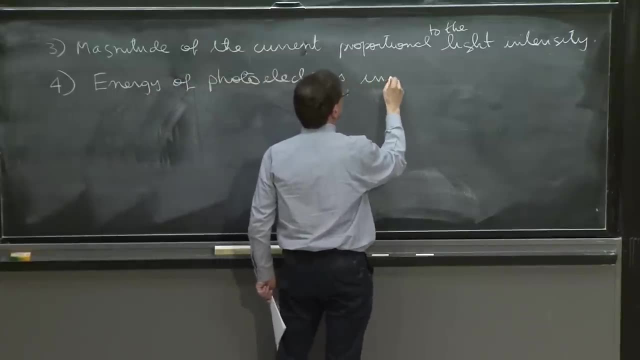 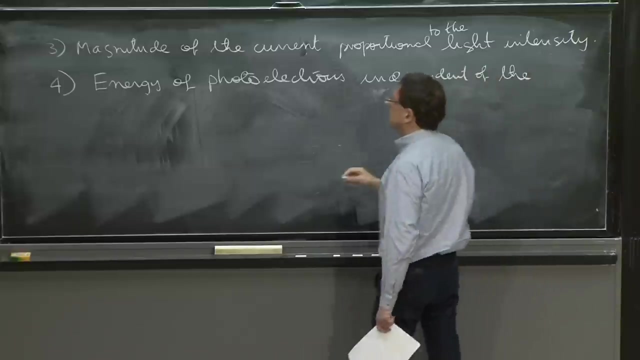 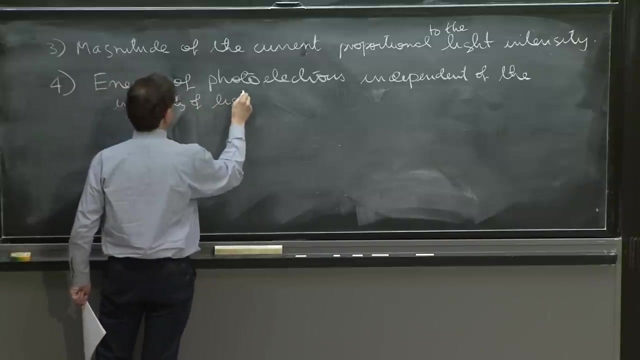 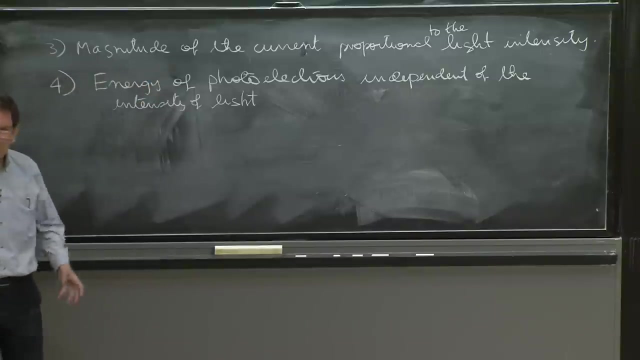 And it seemed to be independent of the light intensity. So energy of the photoelectrons is independent of the intensity of light. The number of photoelectrons would depend on the intensity of light, but not the energy of the photoelectrons. Now there is more to that. 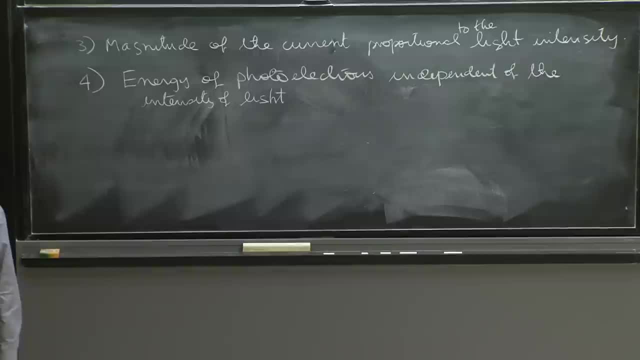 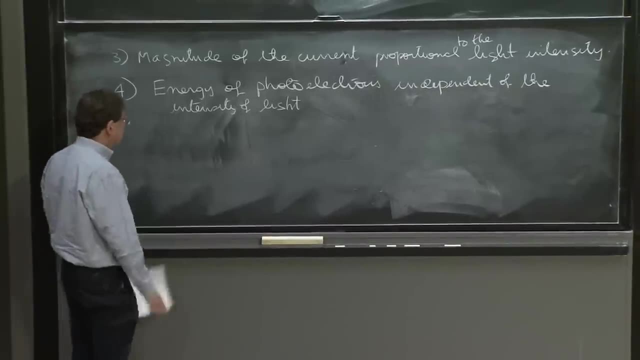 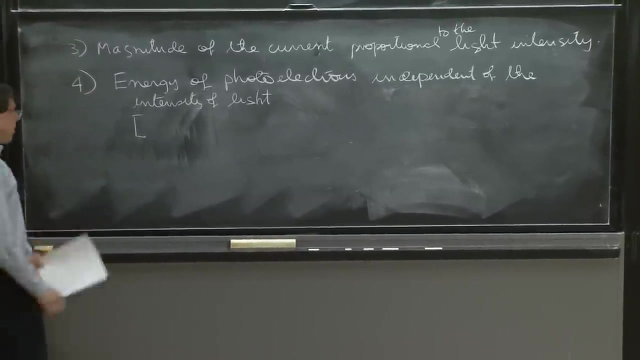 But I think it was not quite exactly noticed by Hertz. So Hertz probably did notice all these things. But the last one that maybe we can put in brackets here is is that the energy of the photoelectrons E gamma. 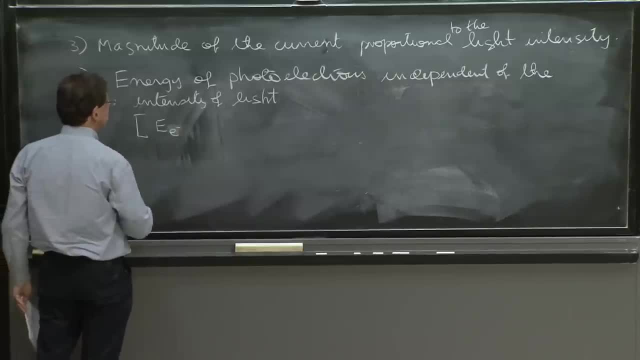 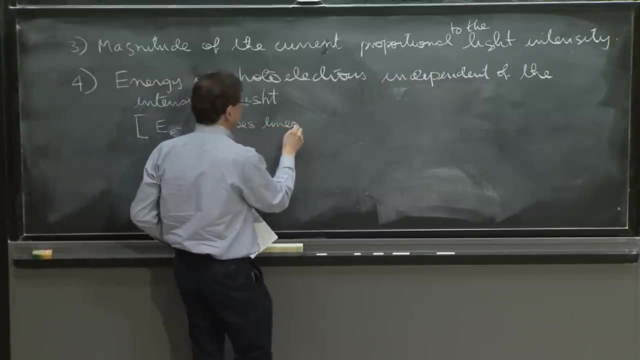 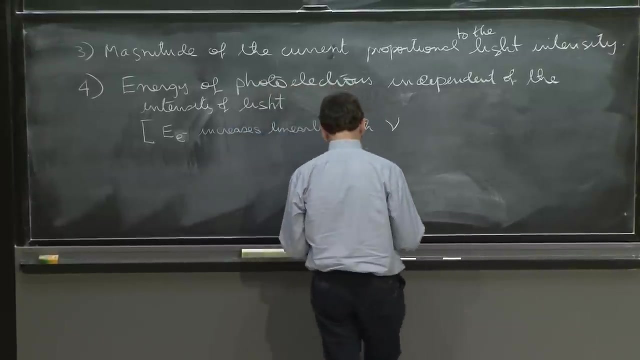 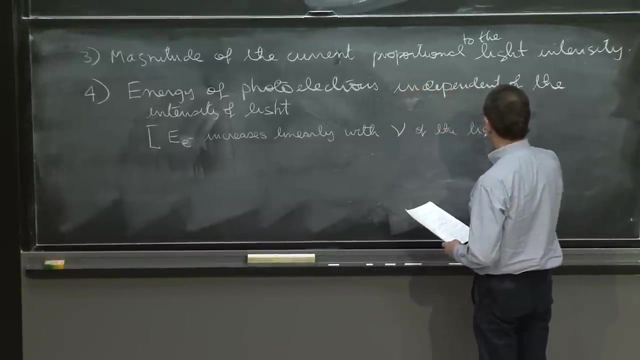 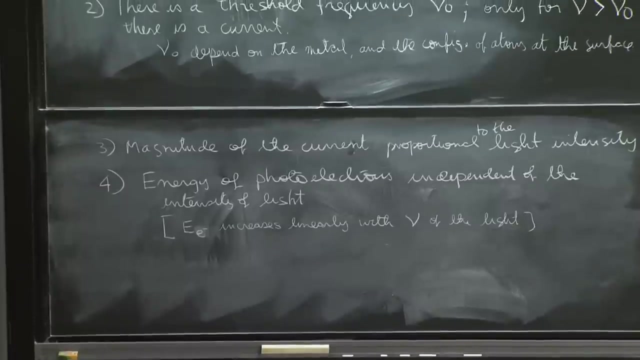 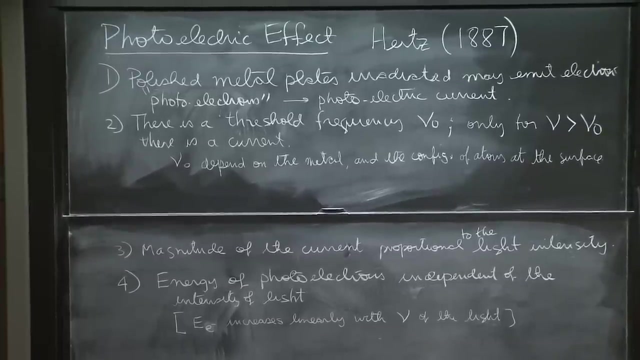 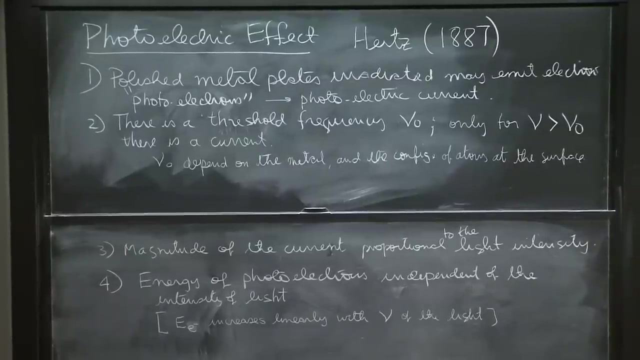 Oh, no, Bad idea. E of the electrons increased increases linearly with the frequency of the light. So this photoelectric effect was not easy to understand if you thought of light as a wave, And Einstein came up with an answer that he almost said what was going on. 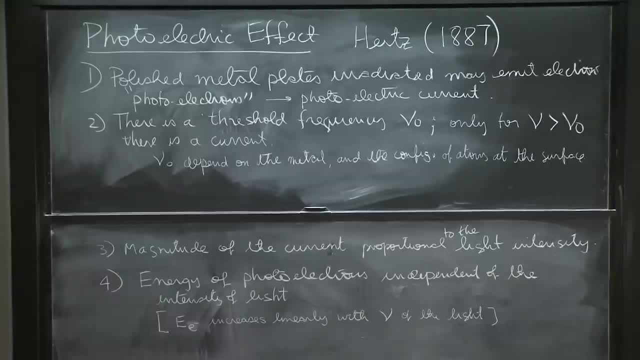 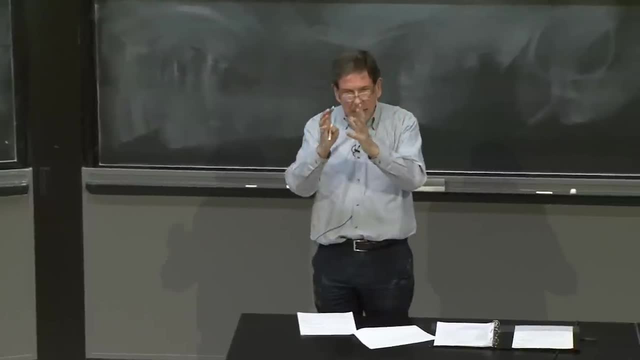 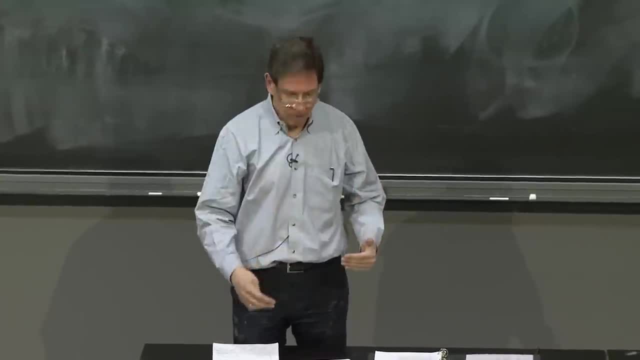 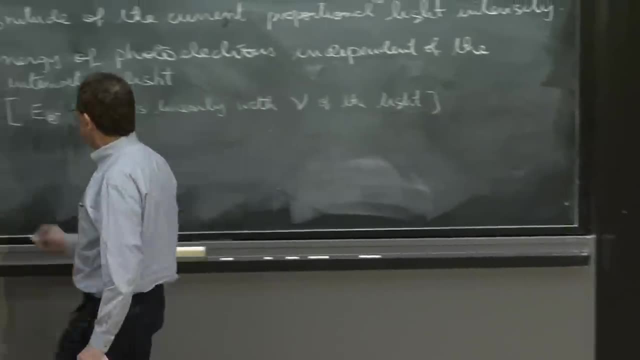 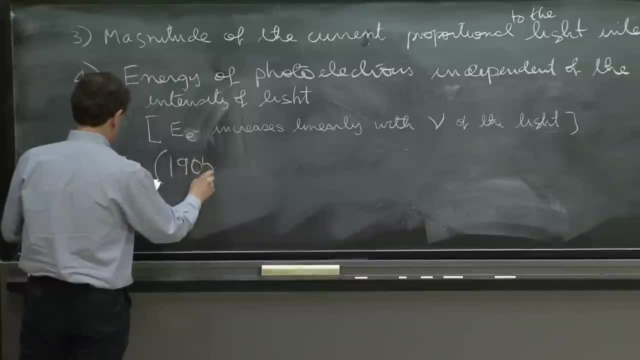 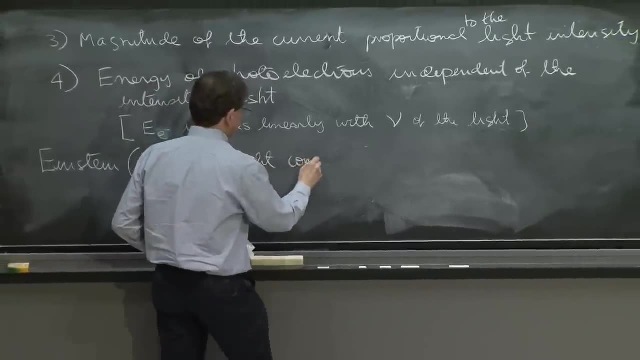 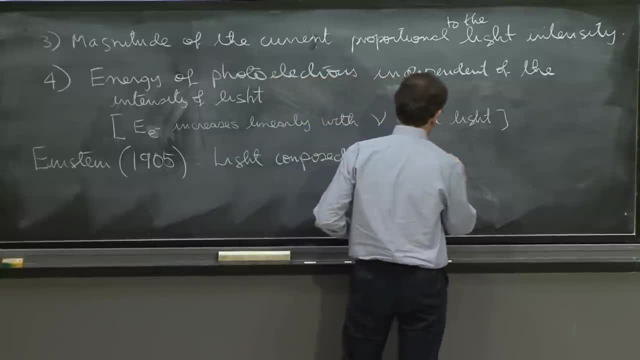 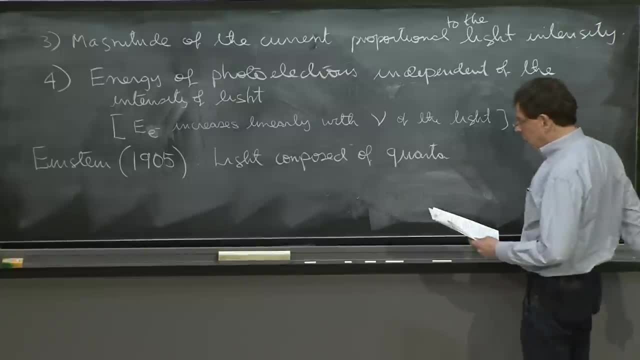 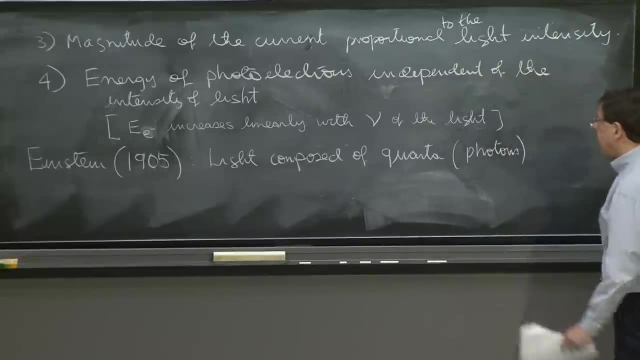 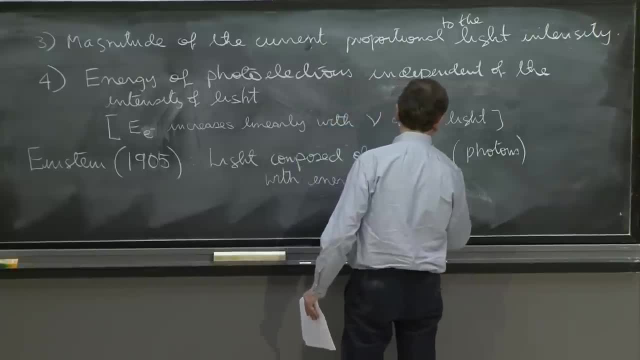 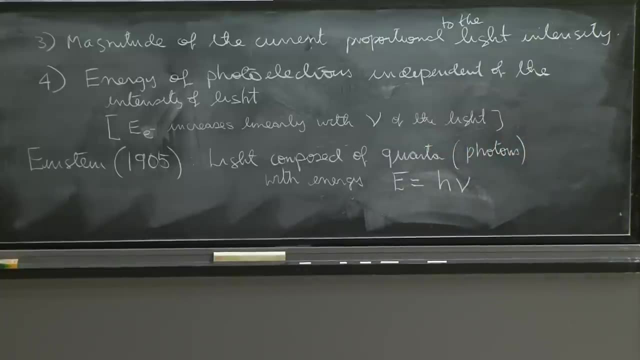 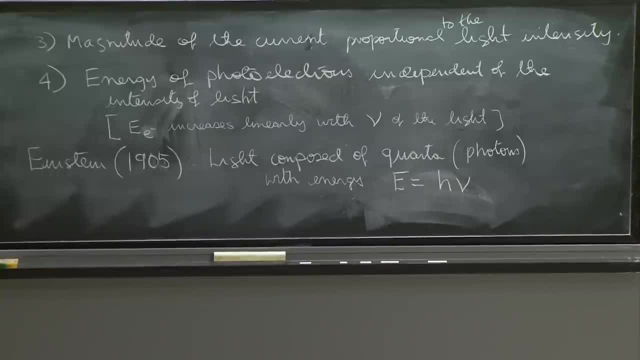 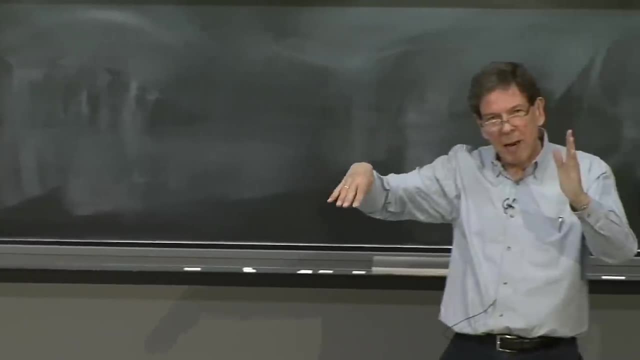 to fit the black-body spectrum. So lots of spacerebbe. LUIS Rograf. The blackbody spectrum, the intensity of light as a function of frequency in blackbody radiation, had a particular curve. Planck tried to fit it. 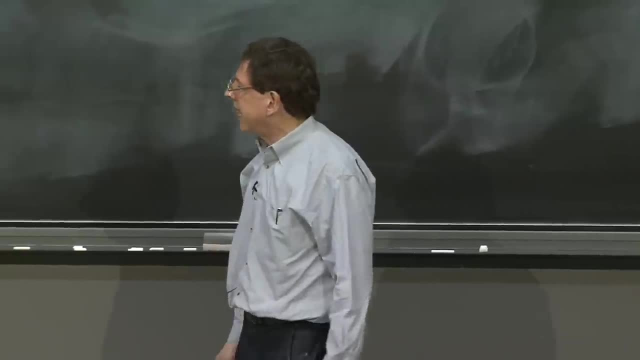 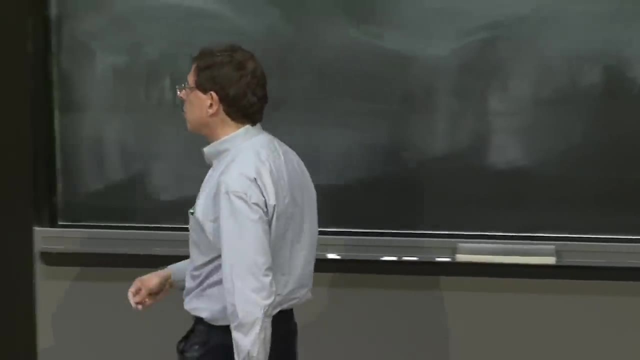 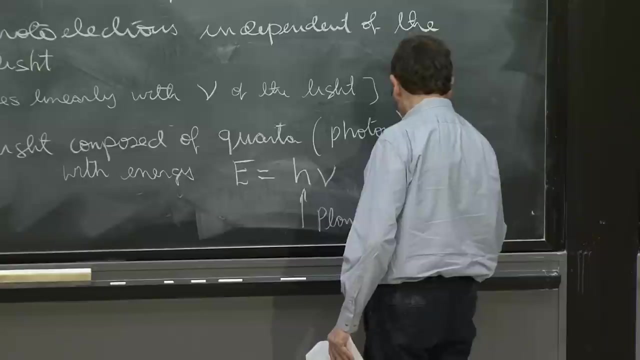 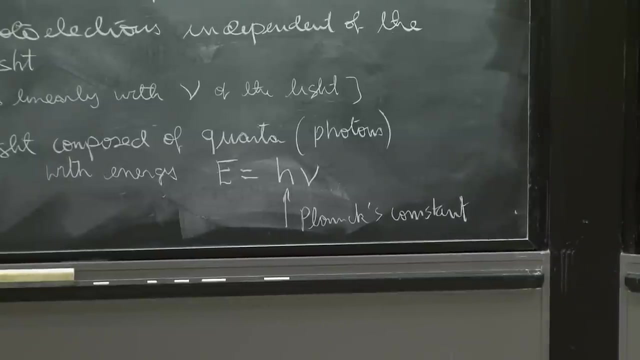 And he realized he needed one constant And he called it h. That's Planck's constant, And the same constant that Planck introduced reappeared in Einstein's proposition. This is Planck's constant. So the picture that Einstein and others had- 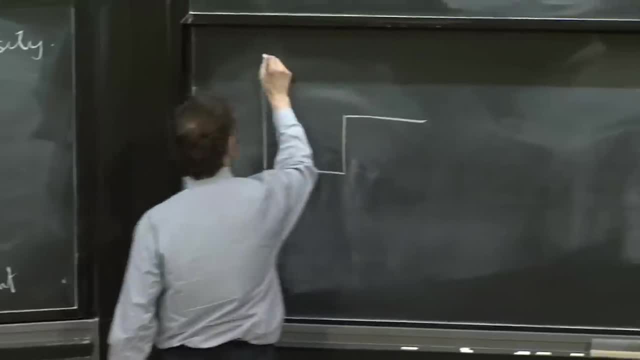 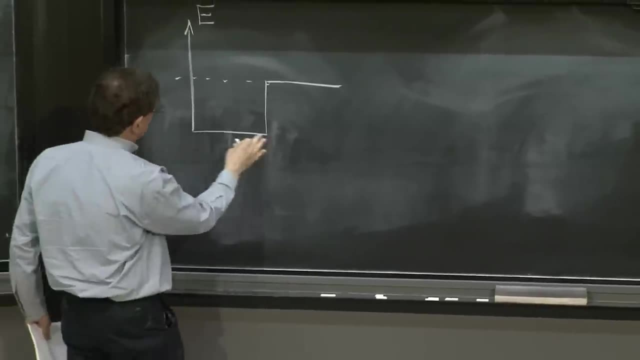 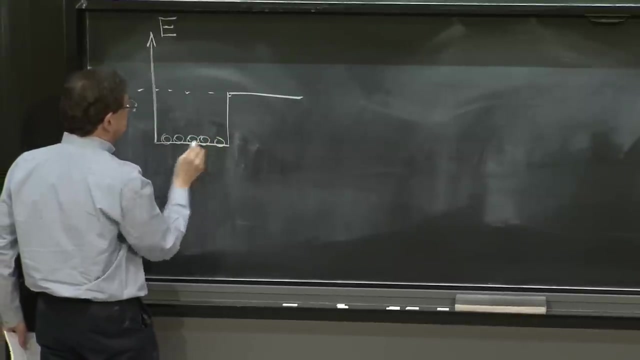 was that you would have a kind of a potential here. You plot energy over here And maybe this is some distance And you have a metal And there's the electrons captured here And here is zero energy. So they have negative energy. 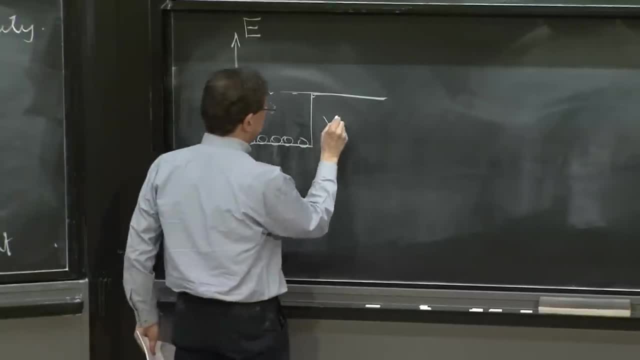 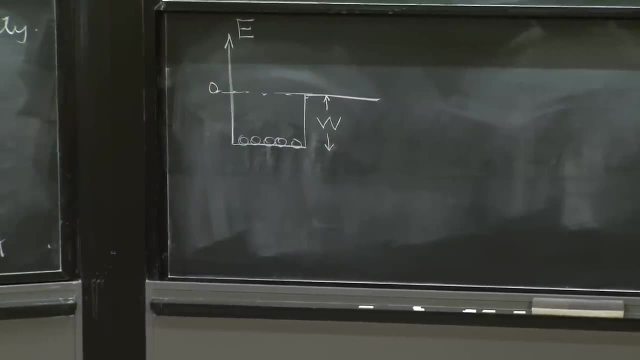 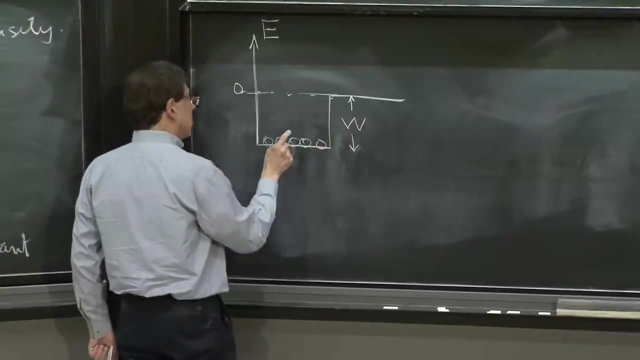 They're captured And you need some amount of energy w, which is called the work function. that depends on the type of metal you have And if you could supply that energy w to any one of these electrons that are bound in this metal. They would come out and not be attracted anymore and would be able to fly free. So this is like an escape velocity: You're bound by the gravity of Earth. You need some velocity, some energy to shoot you out. Same thing here. 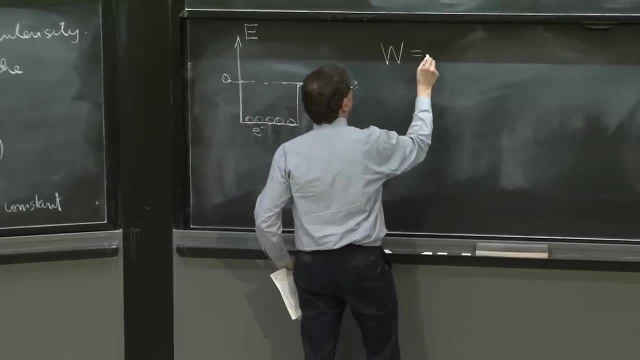 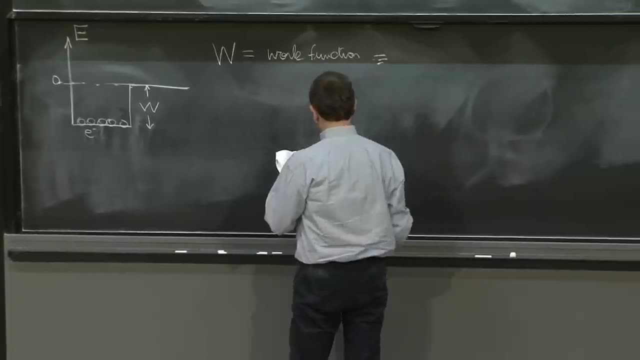 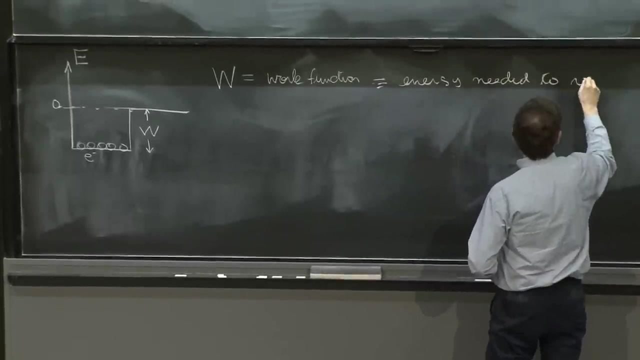 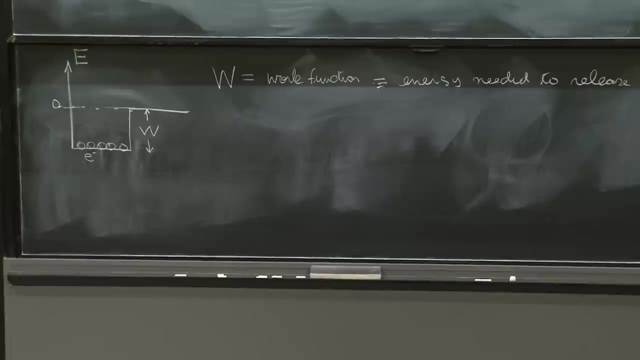 So this w was our work function Function. It's defined as the energy. It's defined as the energy needed to release an electron And that's that work. function is that thing that depends on the metal you have and the structure and how well you've polished the surface. 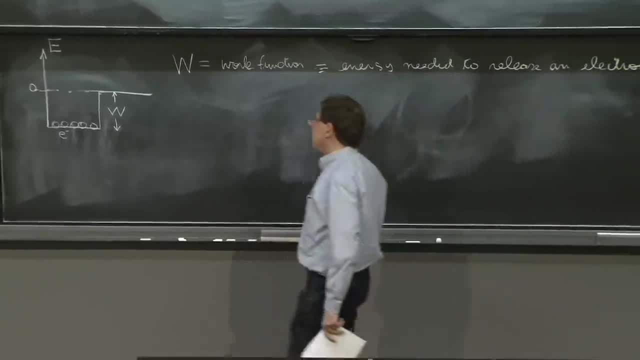 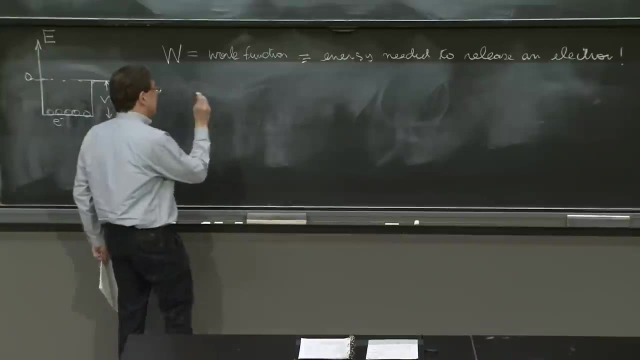 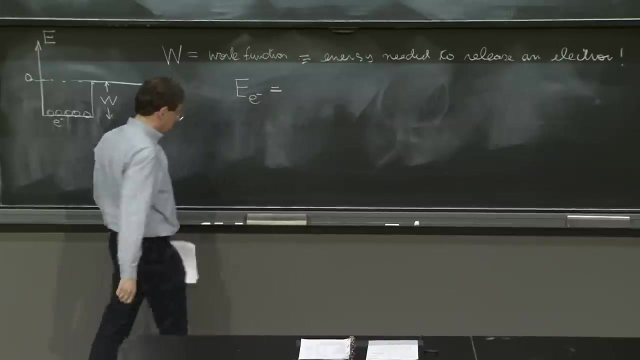 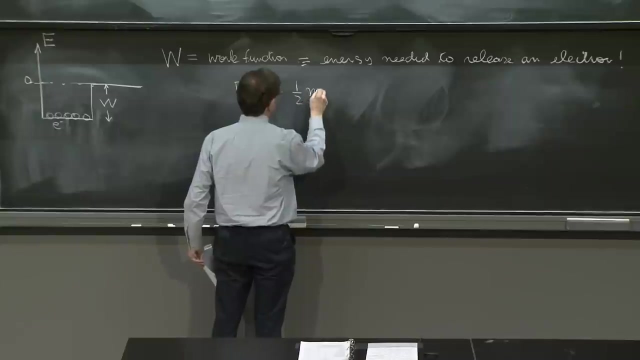 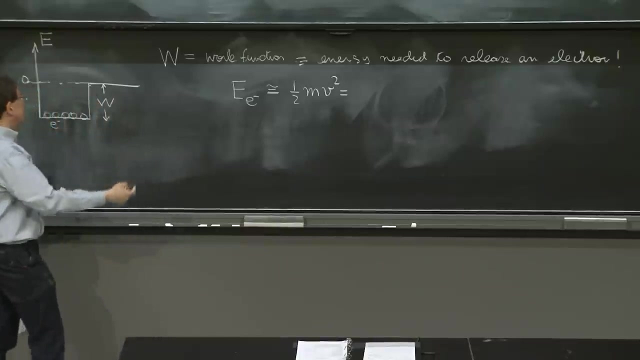 So if this is true, then Einstein, if he, he, he, he, he, he was right with this property, there would be the following statement that you could make: The energy of the electron, which is, roughly speaking, 1 half mv squared, would be equal to the energy that the photon 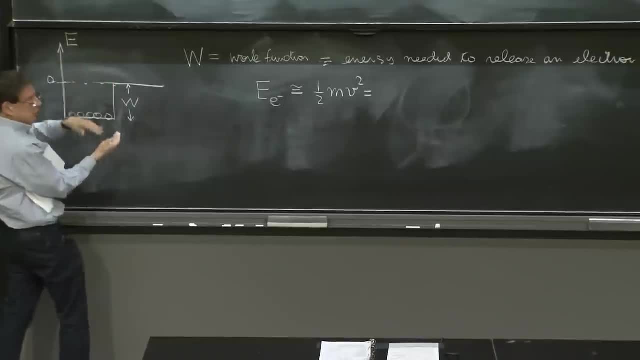 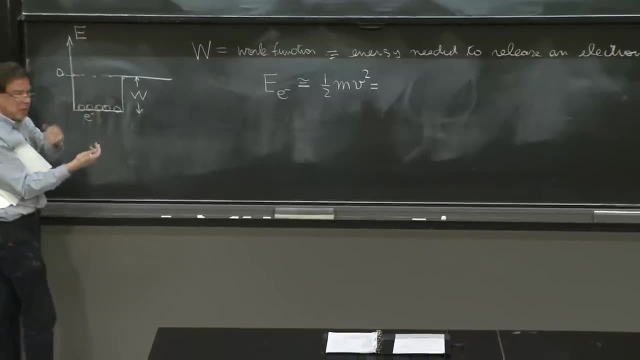 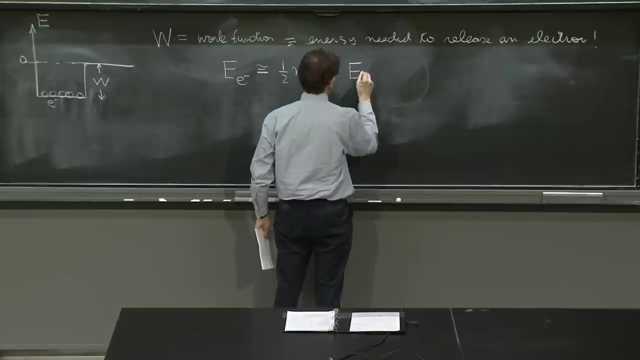 has Minus, Minus, Minus, Minus the work function. So you supply a photon. Some of the energy goes into the work function, But the rest of the energy goes into giving free energy to this electron. So you would have the energy of the photon minus w. 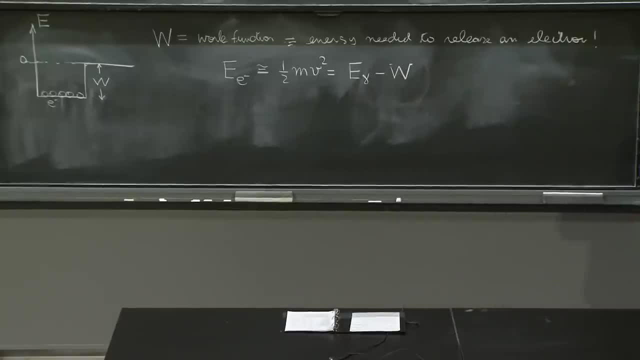 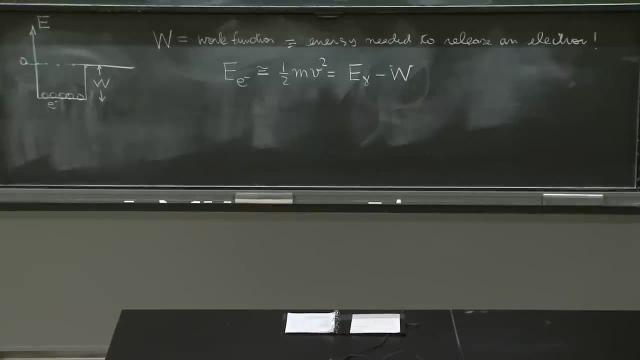 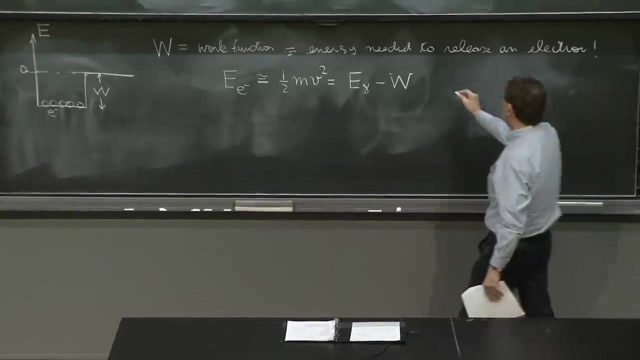 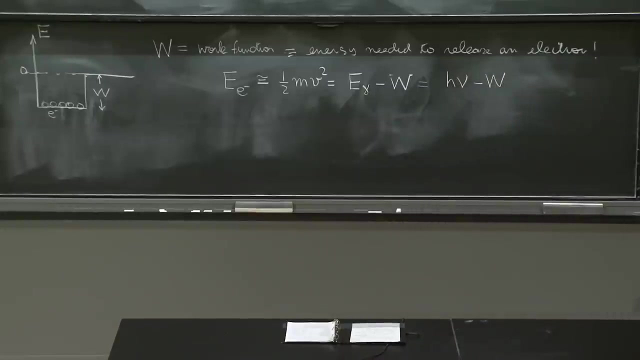 which is what you need to just take it out with zero velocity, And then the rest of the energy of the photon would be transmitted, 可以 the kinetic energy of this electron. So, if this is true, this would be h nu minus omega, And this was considered a prediction. 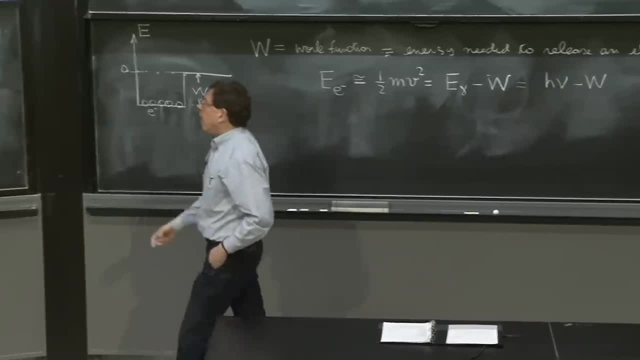 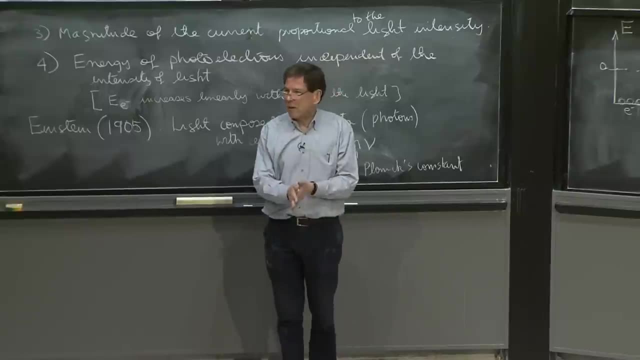 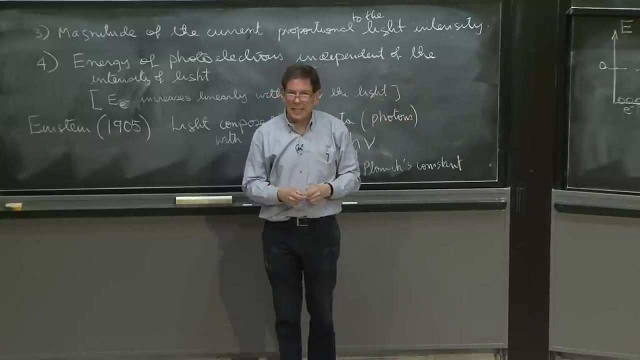 because that statement that the energy of the electron increases linearly with the frequency was not quite obvious to people. Experiments were not fine enough. Measuring the energy of the emitted particles was not all that easy either. So this was Einstein's prediction. 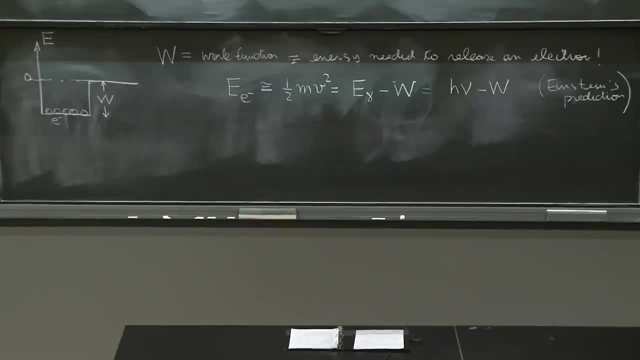 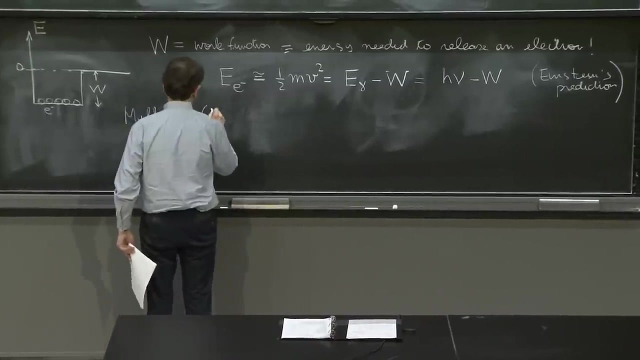 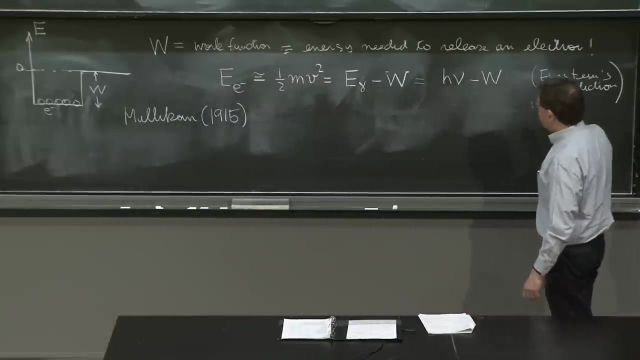 And the experimental confirmation took 10 years to come. It was verified by Millikan in 1950.. So Millikan in 1915, measures the energy of the photoelectrons Varifies Einstein's conjecture. SERGEY BRIZHENSKY, TRUMP, ph, The ads, kimchi. 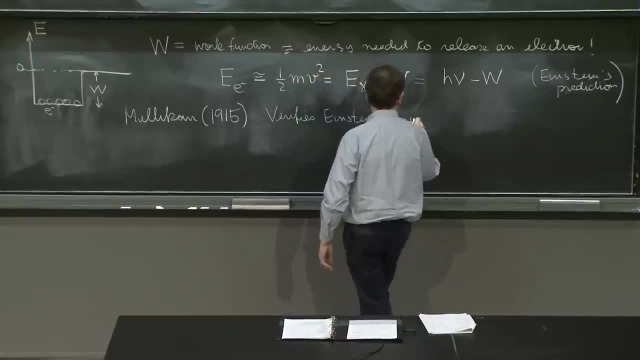 loop pr Right, So tr---- emissions faster expose, so характер. It goes on and on Phil earnings. so I've coveted, over- translated on the where to go. on Jeremiah Bres Bianco reads: a ridiculous experiment. 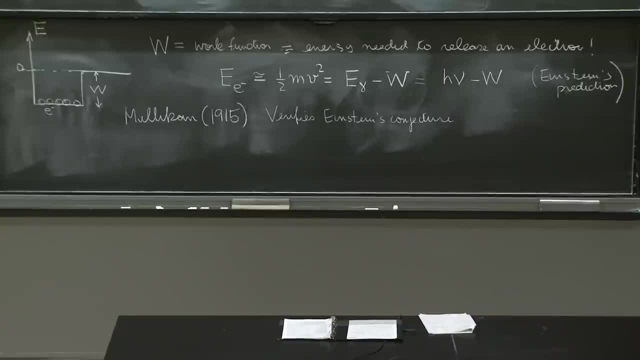 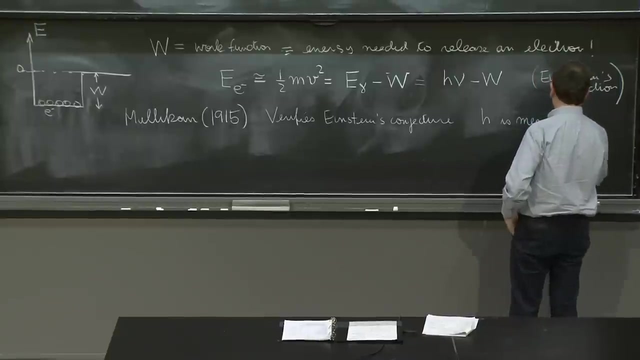 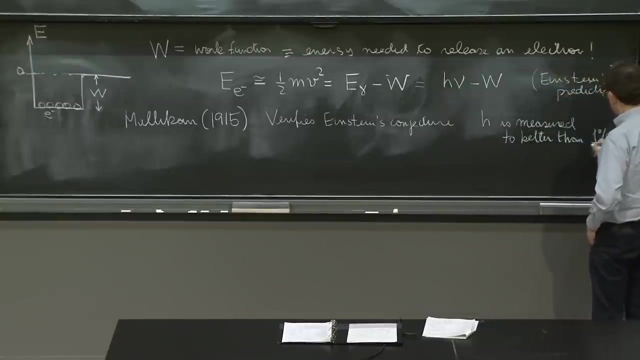 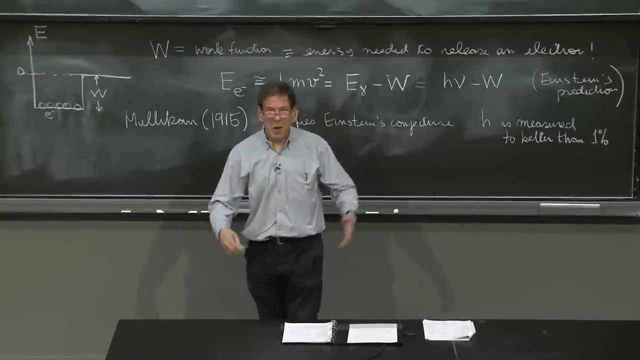 so carefully. the energy of the photoelectrons produces a measurement of h, which is the best to that point, And h is measured to better than 1%. So a very accurate measurement of h, And perhaps you would say, OK, so this is all wonderful. 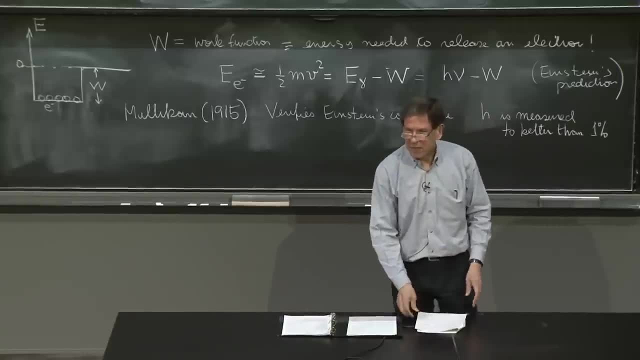 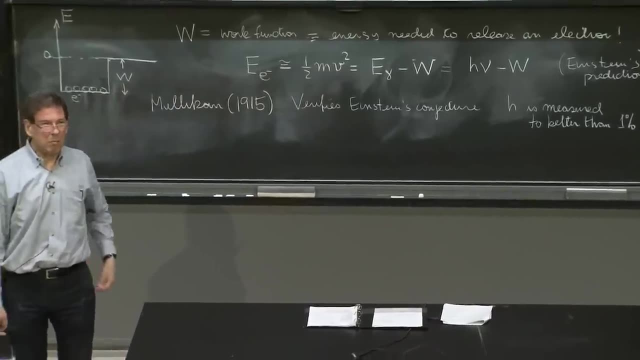 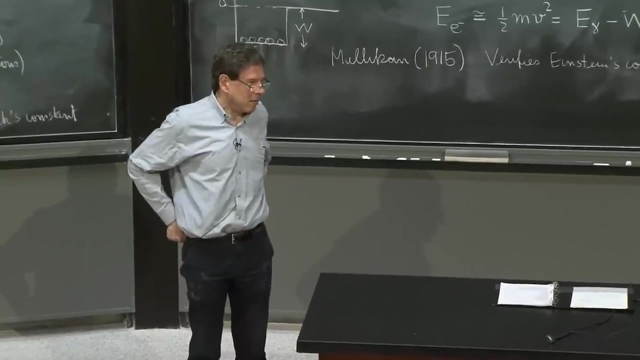 Now everybody believes in photons, But that's quite far from the truth. They didn't believe in photons too much because Maxwell had been too successful And Einstein himself knew that. once you started believing in particles like photons, you had this subject we discussed. 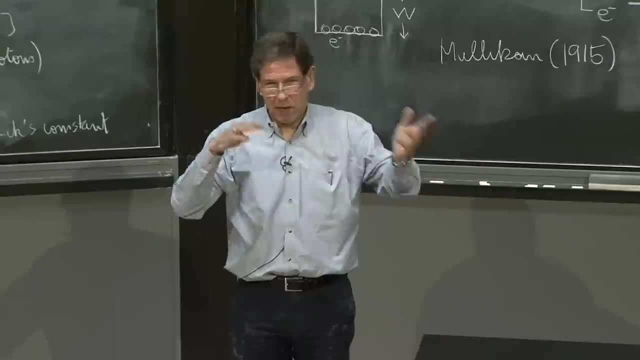 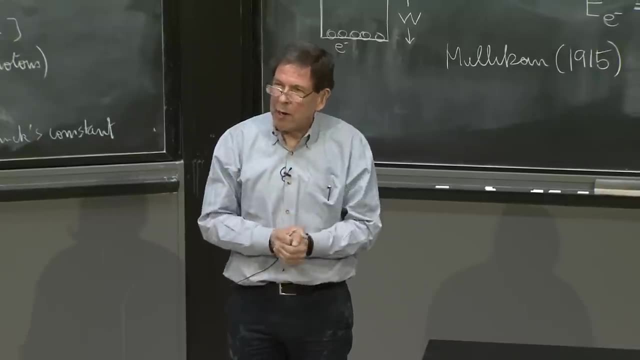 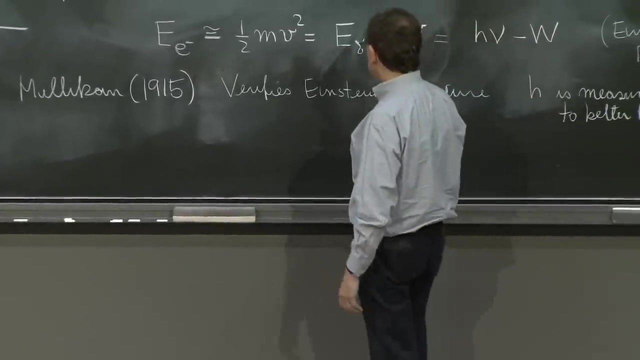 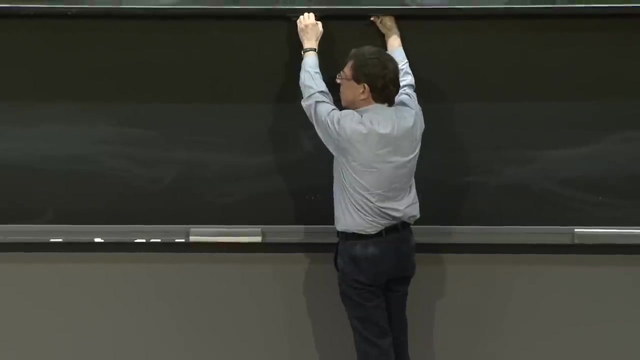 of loss of determinism And waves that behave sometimes as particles, and things he didn't like much, So people were quite reluctant to believe in these things. It's quite amazing. So it took a while still, So let's do a simple exercise to introduce some numbers here. 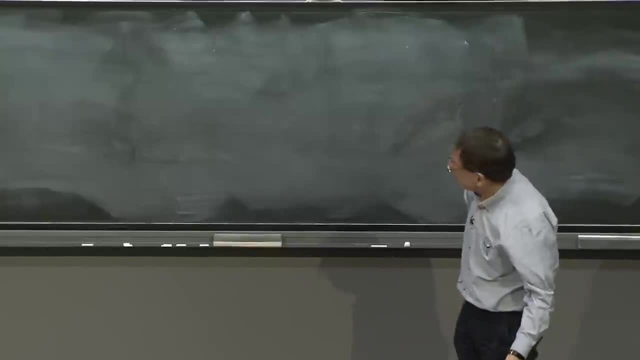 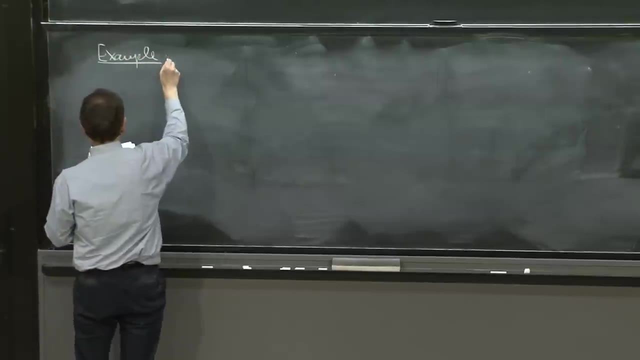 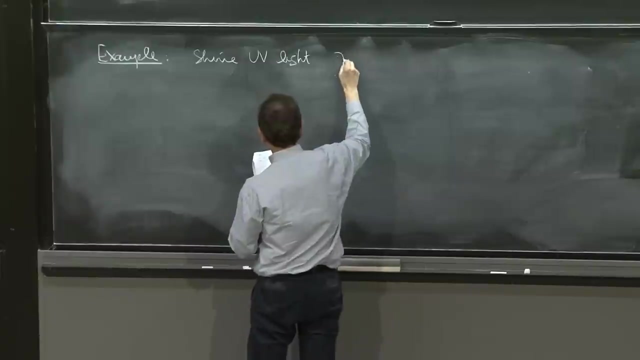 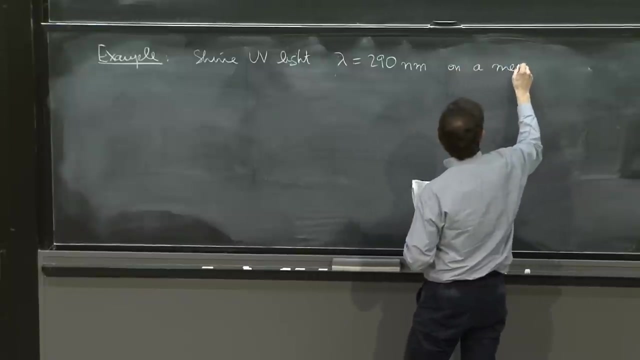 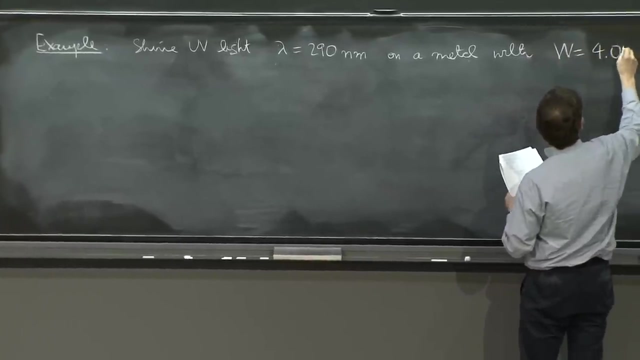 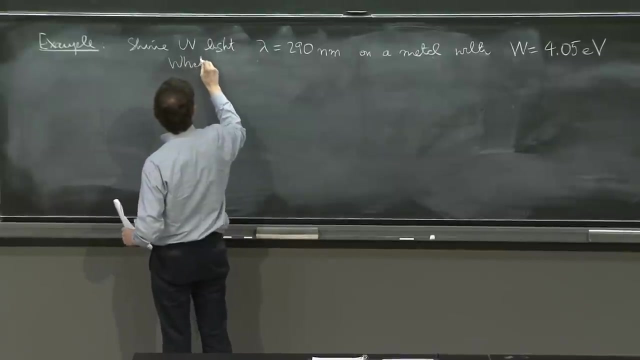 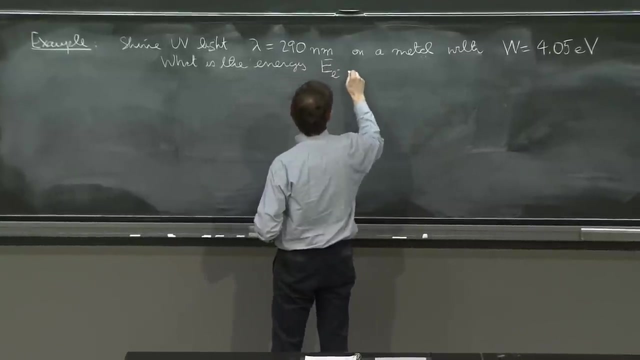 and show you how to do some very simple computation. So let me do an example. You shine UV light with lambda 290 nanometers on a metal with work function 4.05 eV. What is the energy E of the photoelectrons? 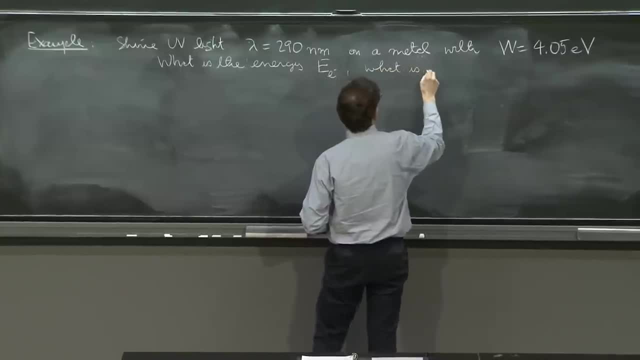 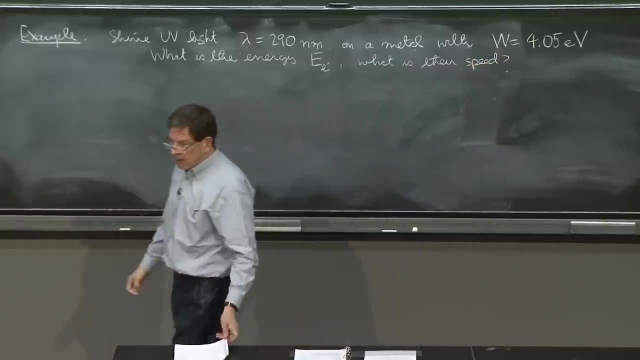 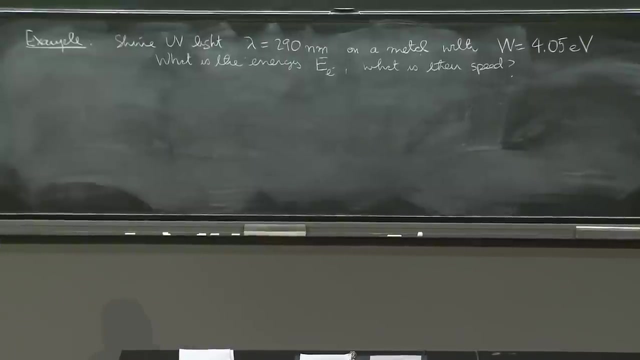 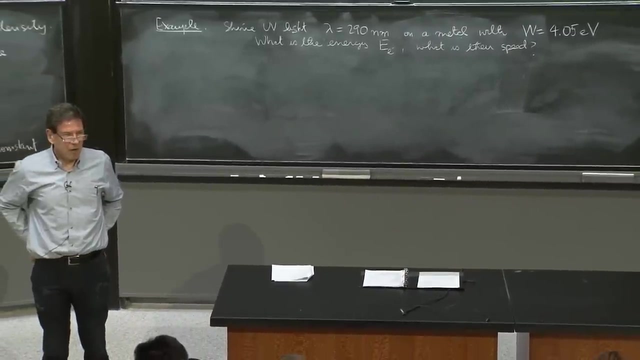 and what is their speed. Now, it is a goal of mine and of the instructors in this course that a calculation like that you should be able to do without turning on your iPhone and checking what the h bar is and getting a few constants and what is an EV. 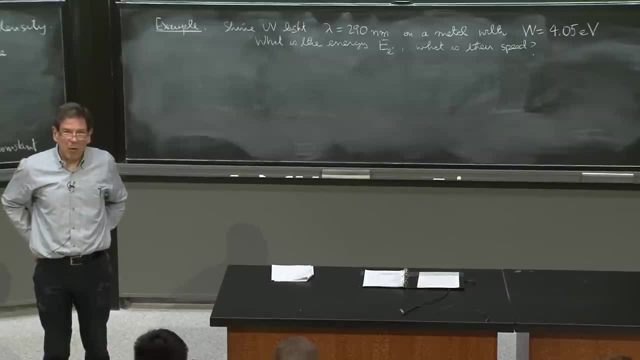 or all these things. Well, nowadays you can just check wall from alpha and they will give you the answer for this in beautiful, beautiful calculations. Just copy the question like that. pretty much I think it will answer. It will answer it for you. 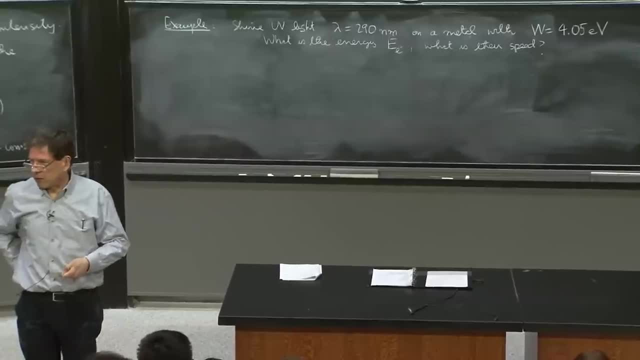 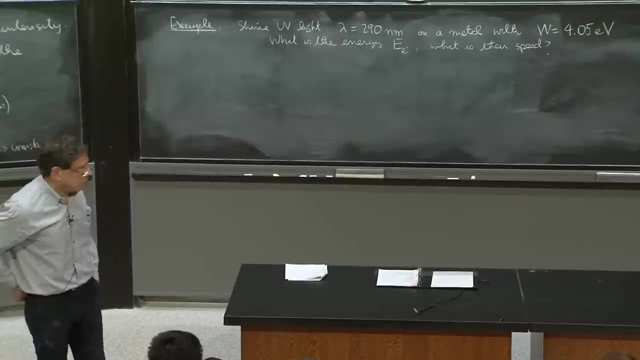 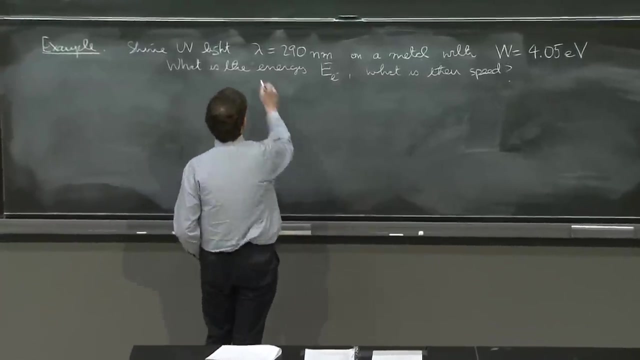 But you should be able to do back-of-the-envelope calculations in which you estimate things quickly And with one significant digit. you don't even need a calculator to do this. So let's see how one does this thing. So the first thing to do is to figure out. 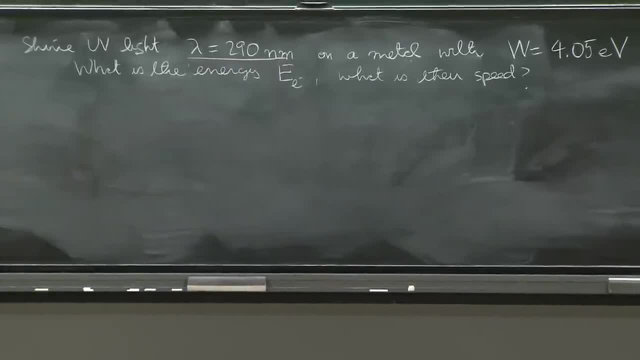 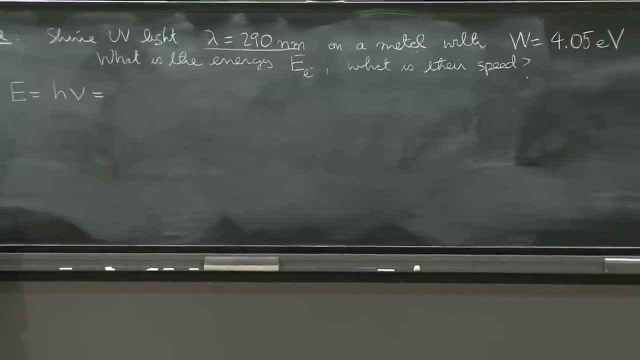 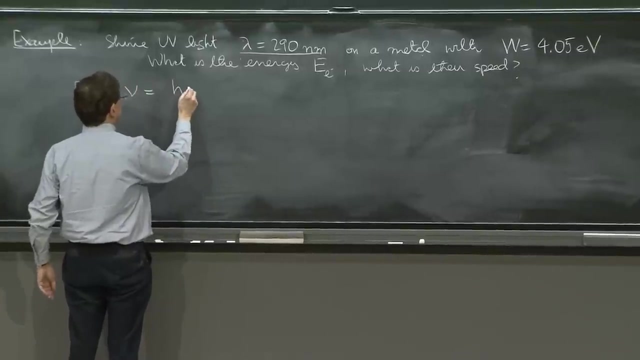 what is the energy of this photon? That's the first problem. So the energy of a photon is h, nu, But nu is not lambda, So nu times lambda is c. So this is hc over lambda, where c is the speed of light. 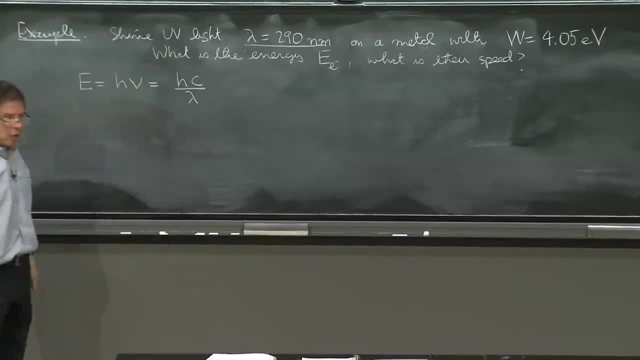 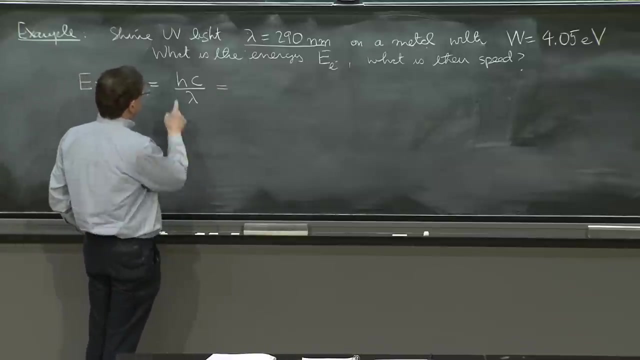 hc lambda. we could do it if we knew h. I must say I never remember what h is in normal units, Joules seconds. 6, point something I don't quite remember. I don't quite remember it. So what do I do? 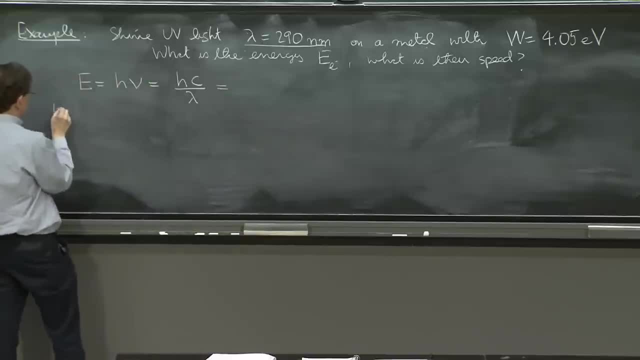 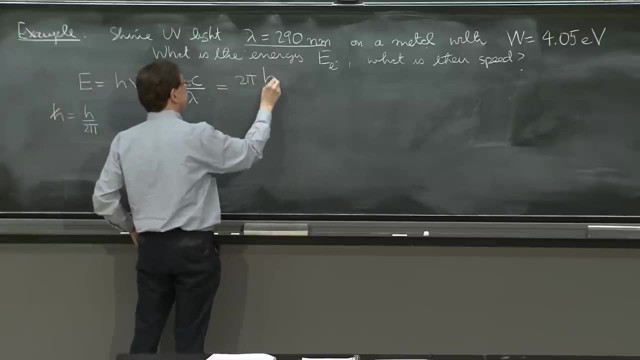 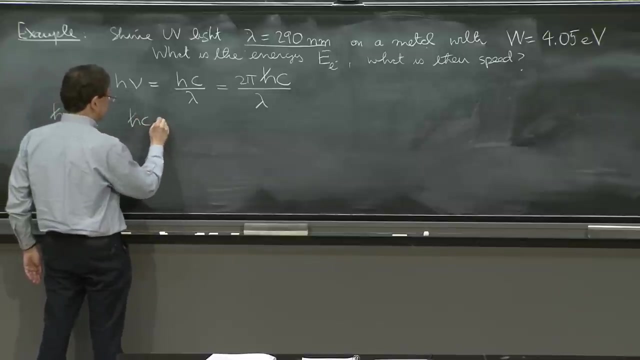 I use h bar, which is h bar is h over 2 pi, So h is 2 pi. h bar c over lambda. And here is where you- here is the first thing that maybe you want to remember by heart. h bar c is a pretty nice number. 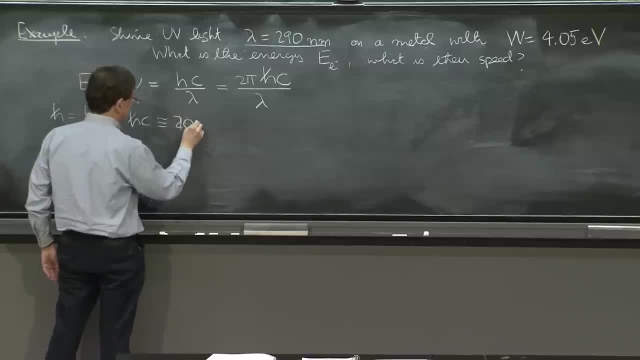 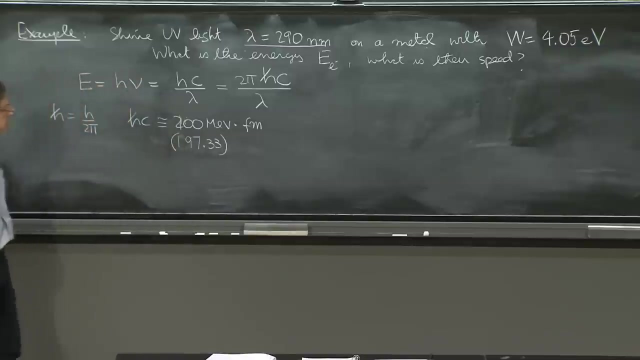 It's about 200 MeV times a Fermi. If you want it more precise, it's 197.33.. If you want to get five digits, But it's pretty close to 200 MeV Fermi And what is a Fermi. 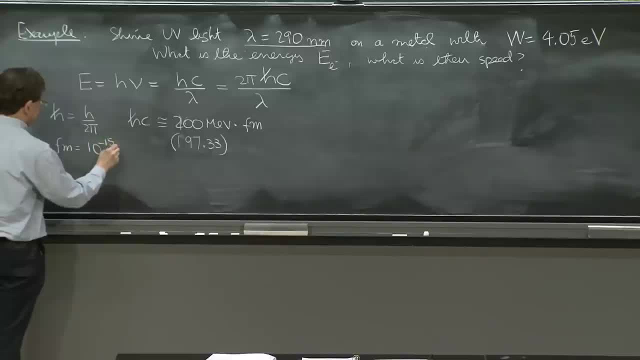 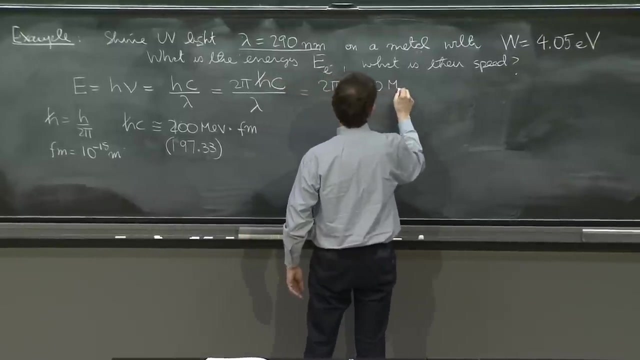 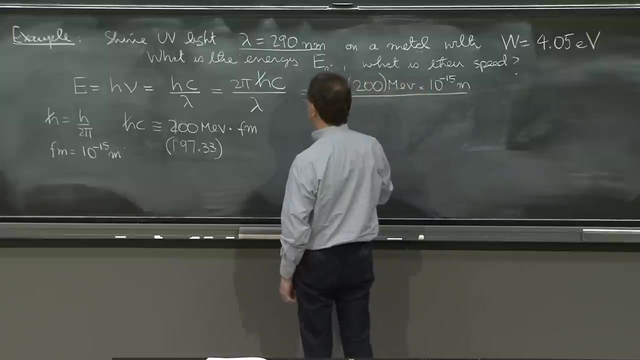 It's 10 to the minus 15 meters. OK, So with this, With this number, I claim, you can do pretty much all you want to do. So here you have 2 pi times 200 MeV times 10 to the minus 15 meters divided. 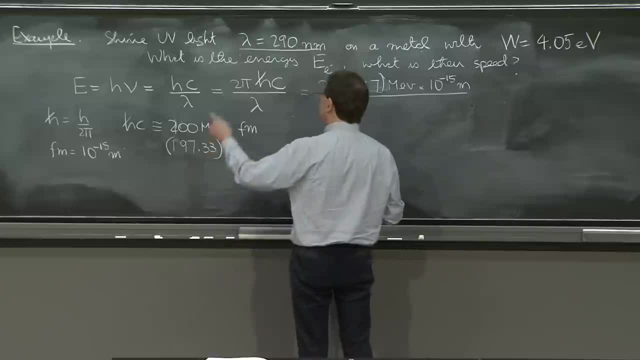 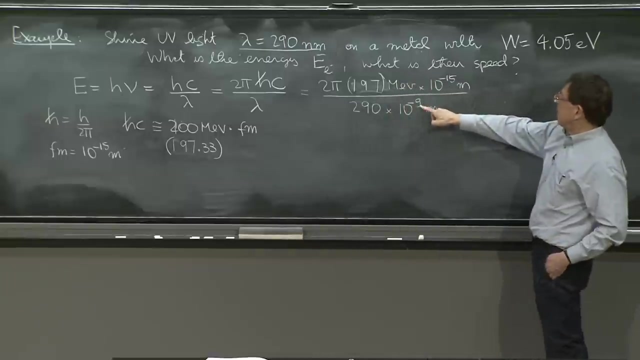 I'll put 197 here: 197 divided by lambda, which is 290 nanometers, which is 10 to the minus 90.. 9 meters, So 10 to the minus 9 and 10 to the minus 15, is 10 to the minus 6 up. 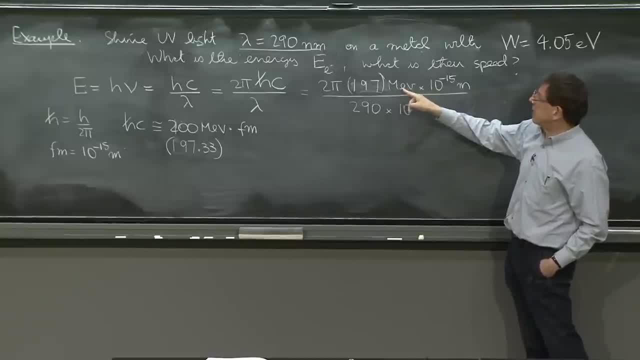 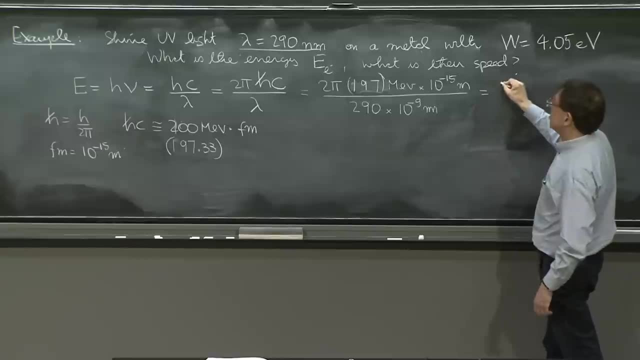 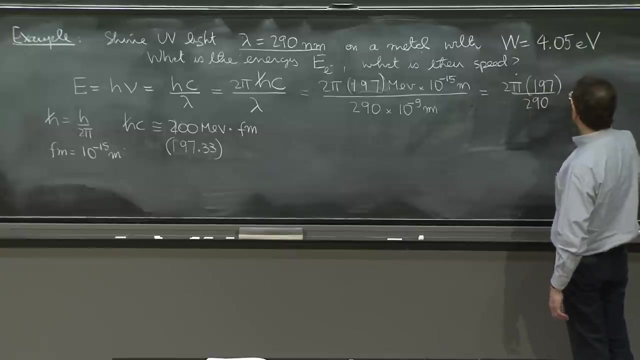 And this is a million eV, which is 10 to the 6 eV. So all these meters cancel and there's just an eV left. So this is 2 pi times 197 over 290 eV, And you certainly can estimate this as like 2 over 3 times 2. 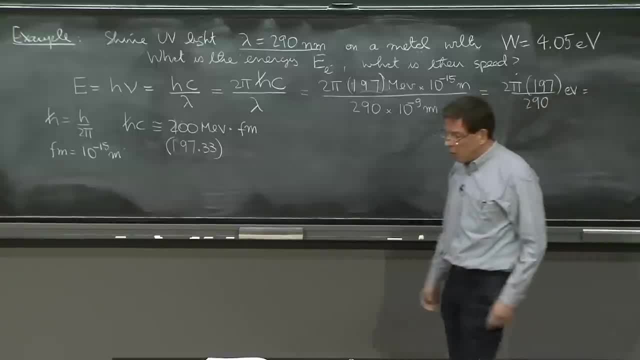 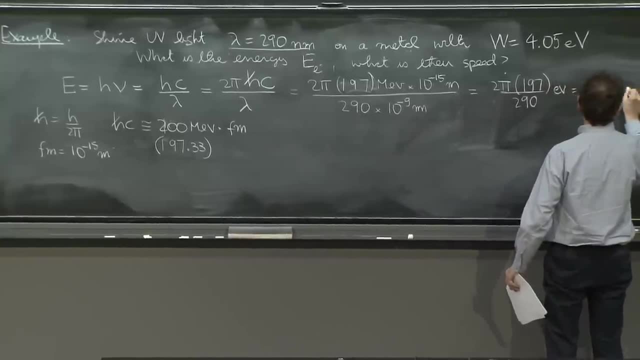 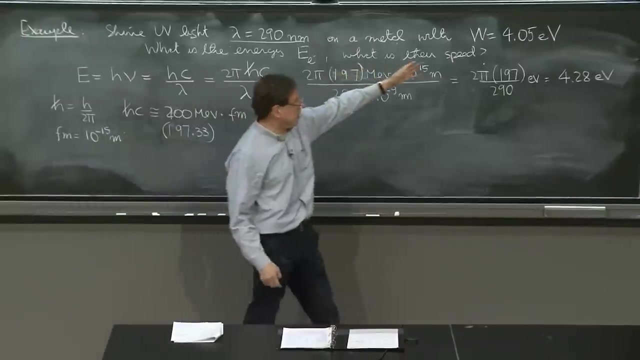 pi, which is 6.. And that's about 4.. And if you want to do it more carefully, it comes out to 4.28 eV. And the nice thing is that the answer comes in eVs And the work functions. everybody gives them in eVs.